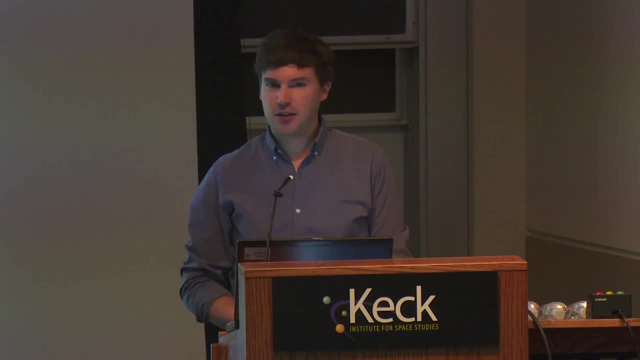 going there someday, But in order to get there, of course, there's many obstacles that need to be overcome, And some of these obstacles we're going to talk about, we're going to hear about today, And one very particular obstacle that needs to be overcome is we need to be able to have 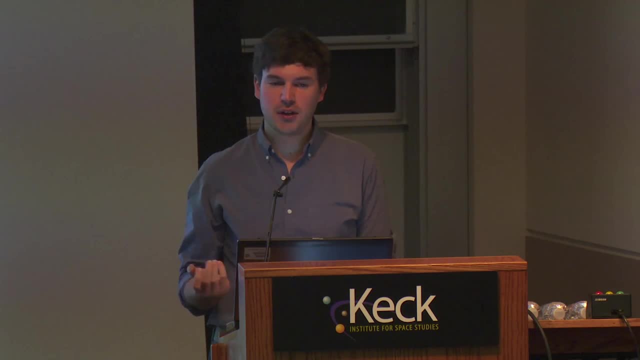 structures on these planetary surfaces or even in space, And these structures must be built Now, of course, on Earth. this is not a big issue, But in order to get up there, we need to send things up there, And most of you may know, but just to mention some rough numbers: to get a pound of material into lower Earth orbit costs on the order of $10,000.. To get it to the lunar surface, it was estimated to be on the order of $50,000 a few years ago, And so if we're thinking of building structures on the Moon or on Mars, 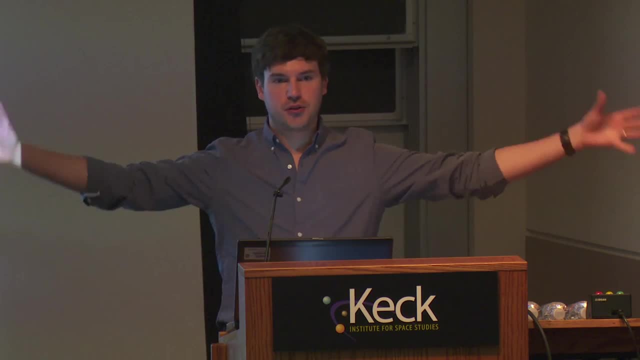 structures are not small precision devices, but structures that are very heavy and very large. We need to do this in a different way, but to send all resources up there, And so the alternative is 3D additive construction, And 3D additive construction really means using in-situ. 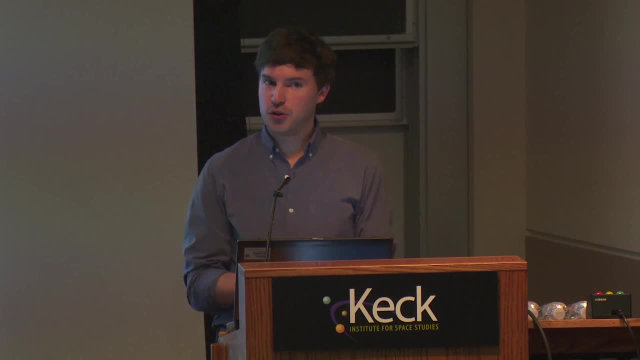 resources, using regolith or whatever can be found on the lunar surface, on the Martian surface, on the planetary surface in general, using those in-situ resources and to build structures with them. But to get there, as we know, many obstacles need to be overcome. 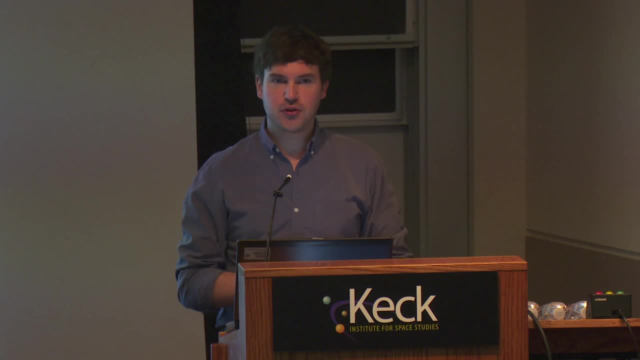 We need new technologies, We need new endeavors in this direction, And this is exactly what this workshop and the short course is about: trying to bring people together who work in the various different disciplines involved in this challenge and trying to see where we can go from here. 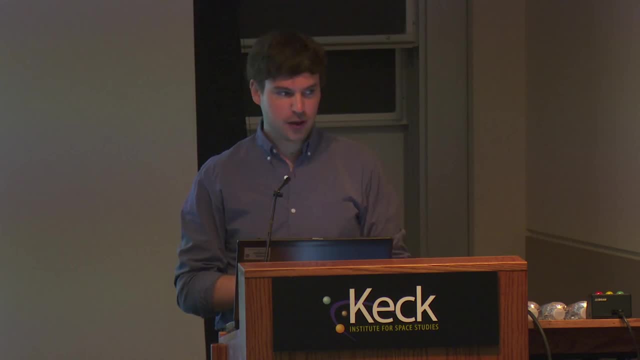 And so, without further ado, I'd like to introduce our first speaker, who's going to be Rob Mueller. Rob is a senior technologist for advanced projects development at NASA Kennedy Space Center. He is in the Exploration, Research and Technology Directorate. He is also the chair of the ASCE Aerospace Division. 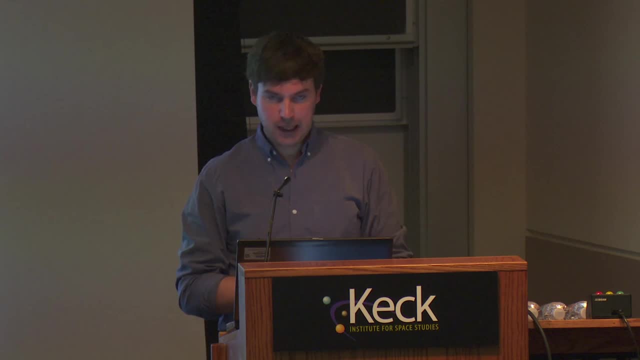 Executive Committee. He was the co-founder of the KSC Swamp Works And he's also the head judge of NASA's annual robotic mining competition for universities. He has been working in this field for quite a while. He's an expert in in-situ resource utilization. We're very glad that he's going to open this morning. 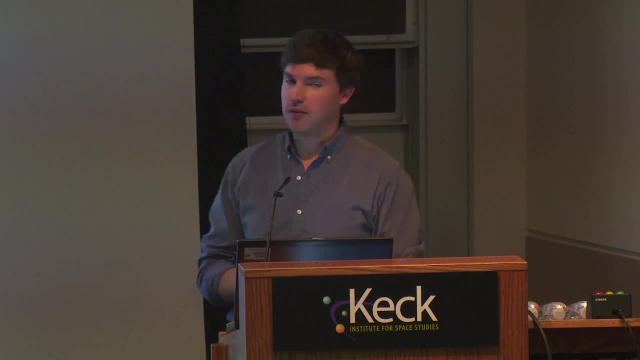 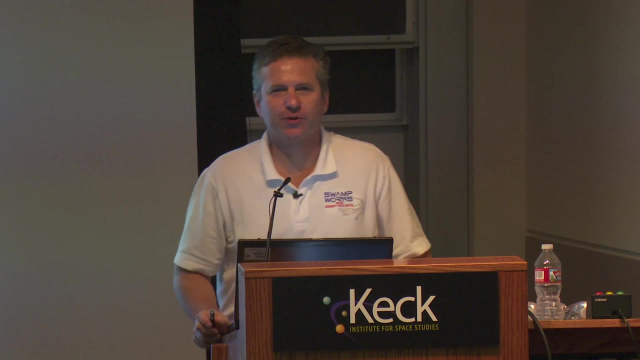 workshop in his first talk entitled Space Environment and Planetary Civil Engineering Basics. Let's give him a big welcome, Let's give him a big hand. Well, good morning. First of all, thank you for coming. We have an exciting topic here today. 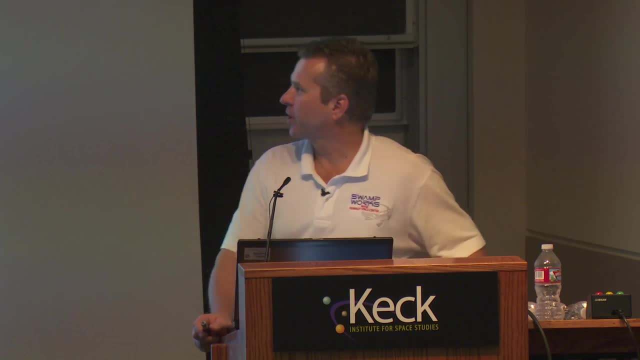 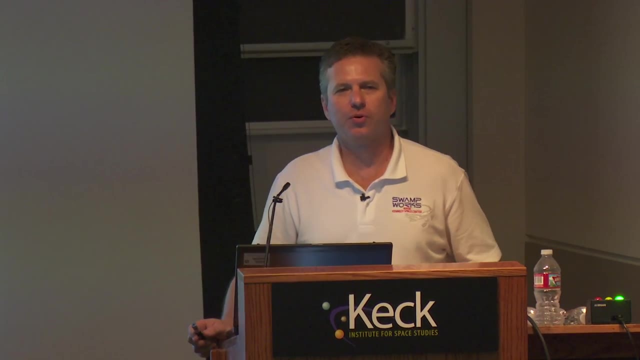 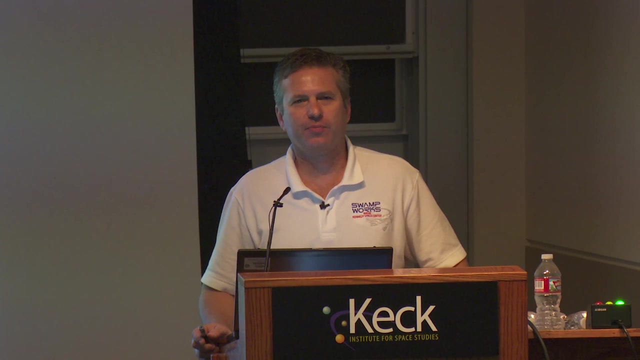 And this truly is new technology in space. What I'd like to talk today is the beginning, the foundations things that you need to know in order to do 3D additive construction in space. So, as you know, this will be very different from anything we're going to do on Earth in the field. 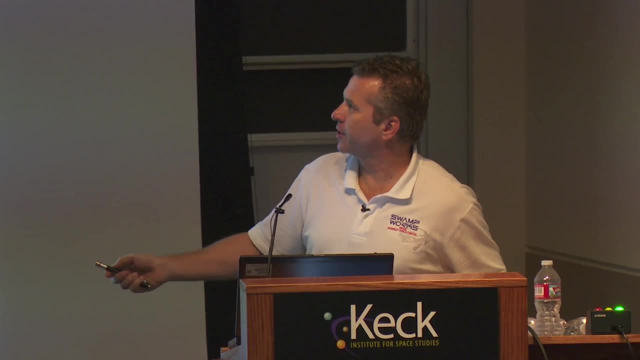 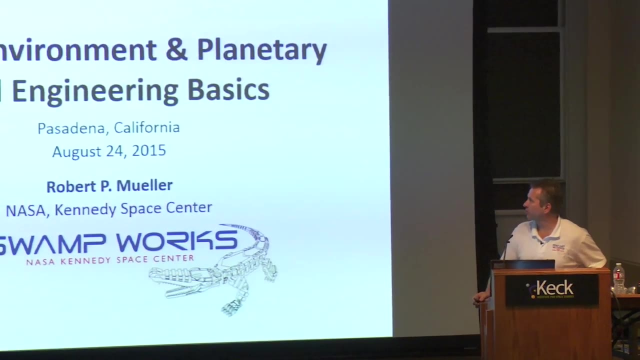 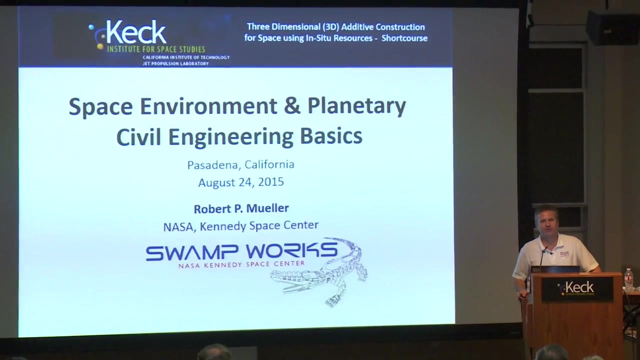 of construction. So the first thing we need to understand is the space environment. What's the environment we're working in? That's completely different from what we have here on Earth. And the second thing is planetary civil engineering basics. Now I'm the chairman of the Aerospace Division of the American Society. 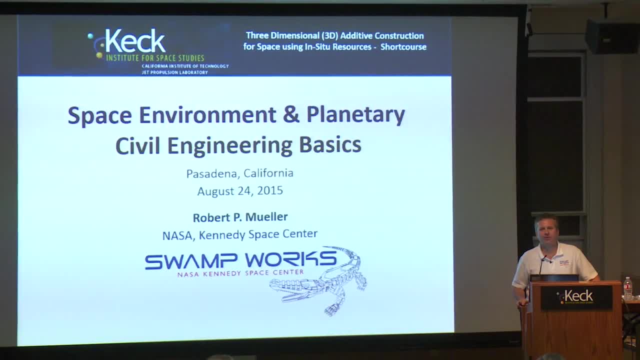 of Civil Engineers, And even when I go to the ASCE headquarters, they always ask me: what are you doing here? Civil engineers don't do aerospace. Well, in fact they do, and they have been doing aerospace for many years, It's just we haven't actually had a mission. 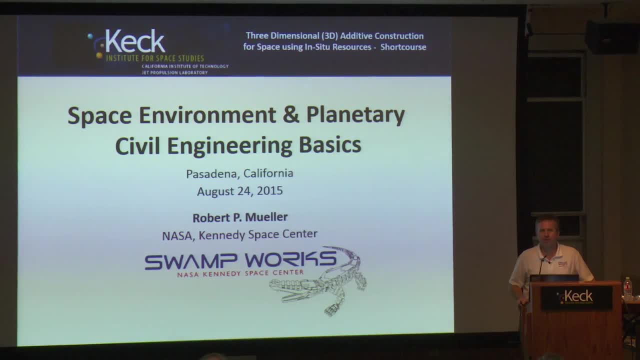 that's done it yet, but there's been a lot of papers written about this subject and we have made substantial progress, at least on the theoretical side. So now it's time to move this into space and actually show how we can do this for real. 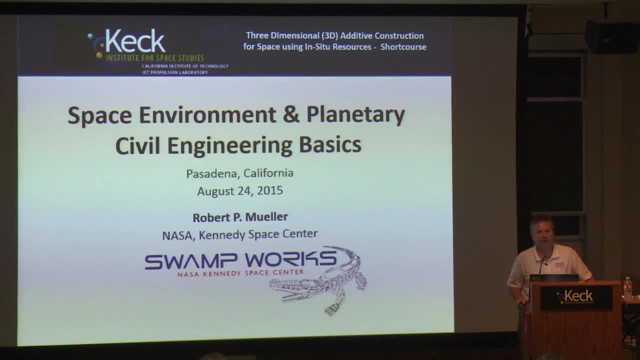 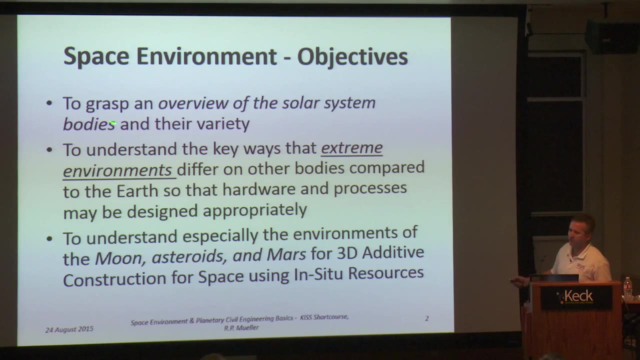 And there's many things coming together at this particular point in time where I do believe we're close to a tipping point where we may see this actually happen. So, without further ado, let's get into the technical side of things. Goal today is, first of all, to understand. 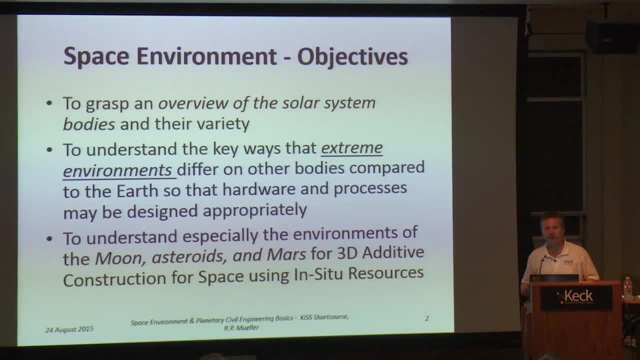 this talk is basically in two parts. The first part will be space environments and the second part will be planetary civil engineering, And I'm going to go very quickly, so hold your questions. for the end, We're going to try to understand the solar system. 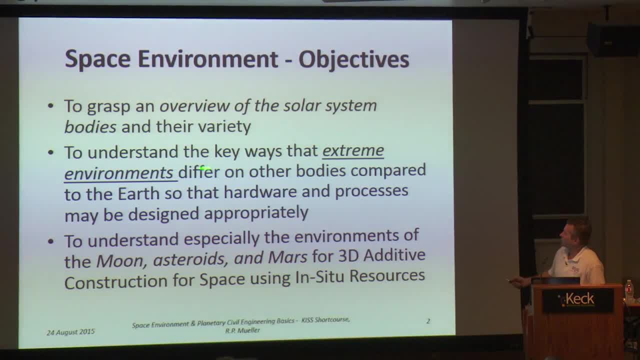 the bodies that are out there and how they can be useful. These are extreme environments and the extreme environments they're different on other bodies compared to Earth. So the hardware and processes they have to be designed appropriately. And notice, I said appropriately. 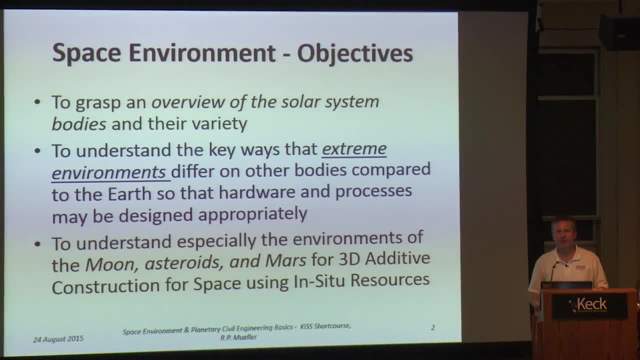 In some cases, we're going to downgrade the strength of materials. In some cases, we're going to use mongrel materials, materials that are actually not as good as what we would have on Earth, but they're good enough. So you have to change your mindset. 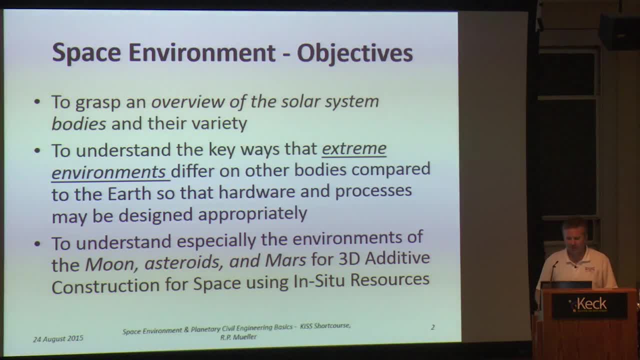 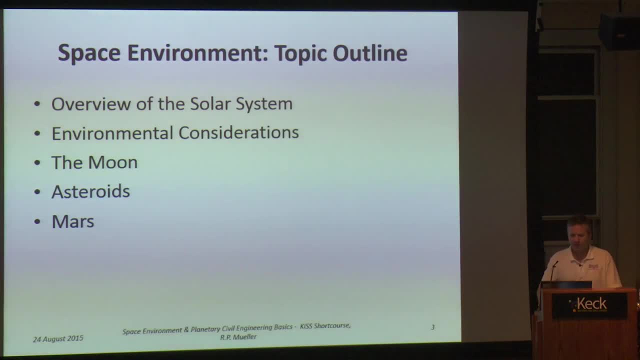 This is appropriate technology, But especially we'll focus today on the moon, asteroids and Mars, because that's the next step and I don't want to get too far out into the future. So first I'll talk of an overview of the solar system. 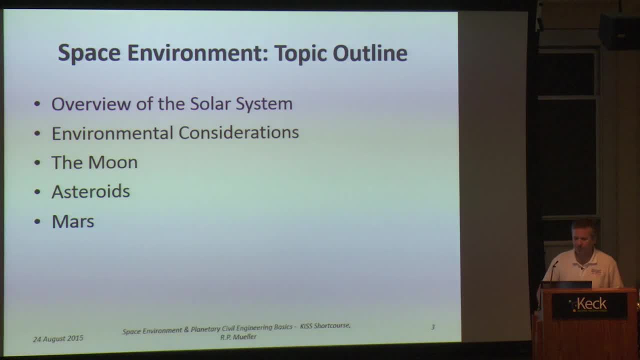 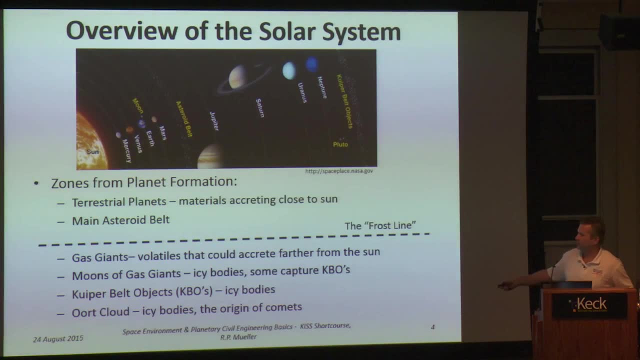 environmental considerations, then we'll talk about the moon, then we'll talk about asteroids, then we'll talk about Mars. So here's the solar system And we basically have this frost line. Now I know you're all a very smart audience. 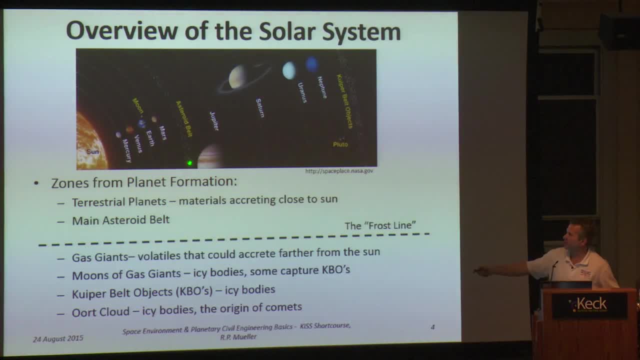 so you know already where this frost line is. The frost line is at the asteroid belt, And that is a unique line, first of all because that's what's feasible today for human space flight, that's realistic, And second of all, it's related to resources. The resources inside the frost belt have a potential for liquid water And the resources outside the frost line have more water, massive amounts of water beyond the frost line. but it's in the solid phase. it's not in a liquid state, so it's harder to use. 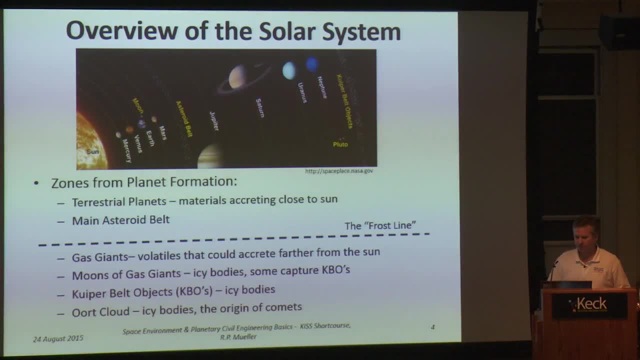 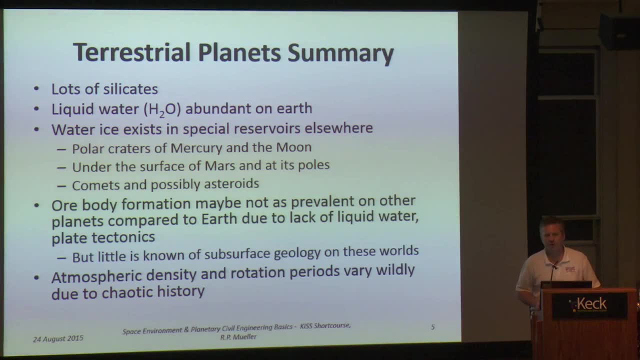 If we go to the inside the frost line, we call that the terrestrial planets. So I'm going to focus on just the terrestrial planets. We're not going to talk about anything beyond the frost line. The terrestrial planets have lots of silicates. 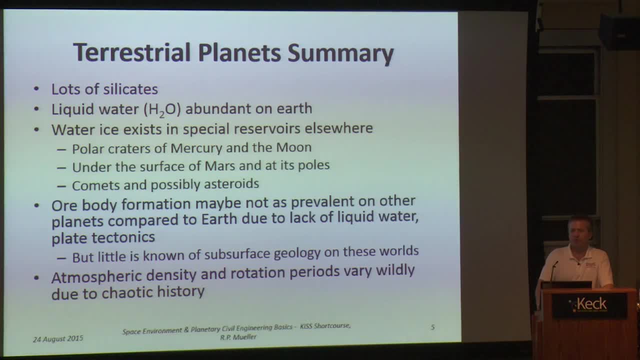 Liquid water is abundant on Earth. Water ice exists in special reservoirs. We have found out that on the Moon, at the poles, there are substantial amounts of water ice. One little calculation shows that there's enough water ice to make propellant hydrogen and oxygen. 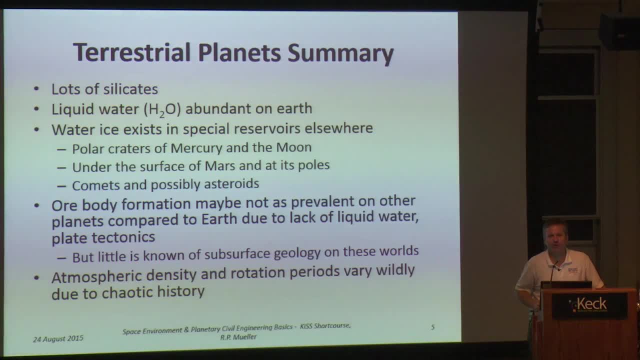 to launch something like the space shuttle every day for the next 2,000 years. Just to put it in perspective, there's a lot of water ice suspected to be at the poles, at the poles of the Moon. We also know there's water ice on Mars. The Phoenix mission showed us that and other missions. And there's even polar craters suspected of having water ice because they're in permanent shadow on Mercury, which is very interesting. The ore body formation is different than on Earth. There's a lack of liquid water and lack of plate tectonics. 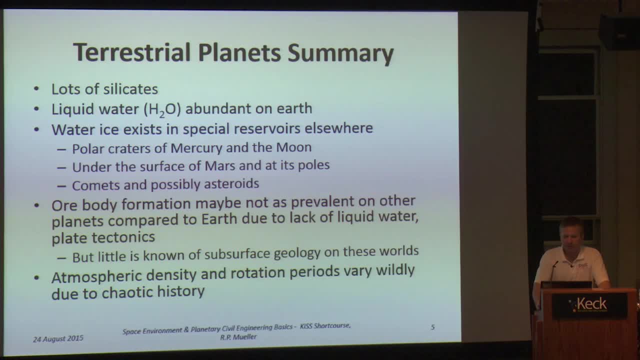 so little is known about the subsurface geology on these other worlds, And the atmospheric density and rotation periods vary wildly due to the chaotic history of the solar system. So we have to accept that every planet is different and that every environment is different. 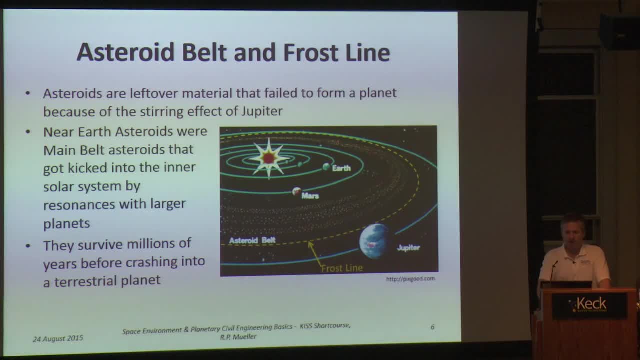 It will not be. Earth-like Asteroids are leftover material, So if in the beginning of the solar system this was a violent event And so there were many asteroids formed, There's a large quantity of asteroids in the asteroid belt and essentially it's debris. 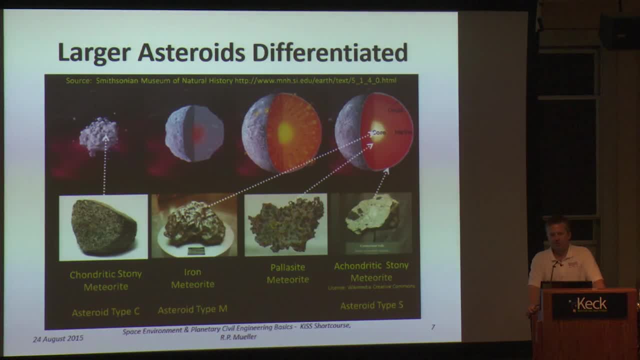 And this debris is formed into planetary bodies that we call asteroids, And they can be made of chondrules and then they form these chondritic asteroids, Or they can be actually small bodies that have differentiated and then had some kind of violent collision event. 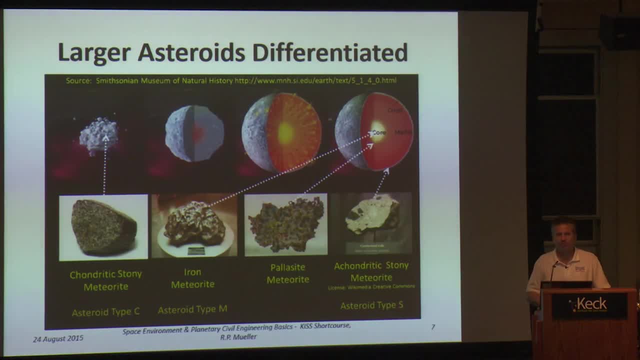 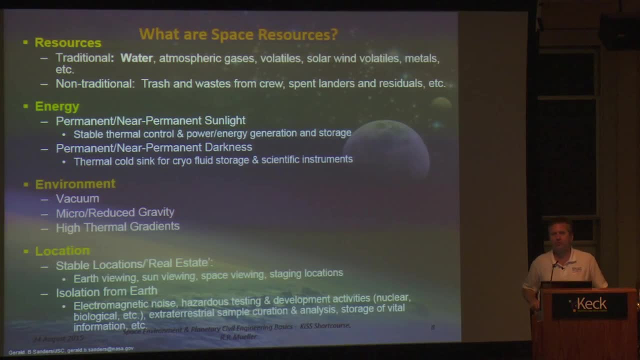 and then split up into these other types of asteroids. So there are many, many types of asteroids out there, which is is good because it gives us access to the resources. One good thing about the asteroid belt is there's no gravity. well, So you don't have to enter or exit the gravity well, And the resources are many times at the surface. You don't have to dig down because they've already. Mother Nature has already broken them up for us. So what are space resources? 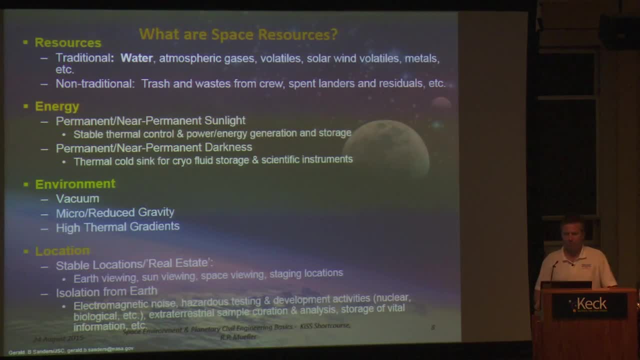 Well, traditionally we talk about water, atmospheric gases, volatiles, solar wind, volatiles, metals. But we've also expanded. it's nothing new, but recently people have started to realize that if you land on another planetary surface, then there's a lot of waste material. just a lander stage. 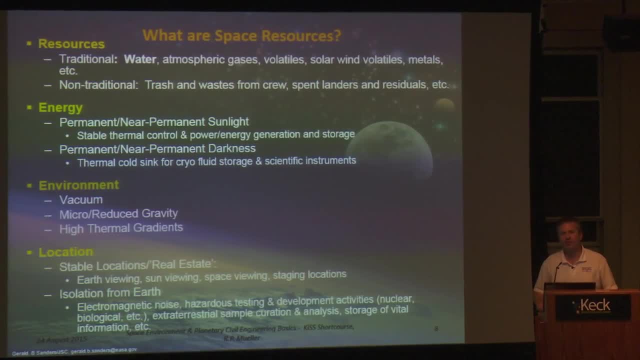 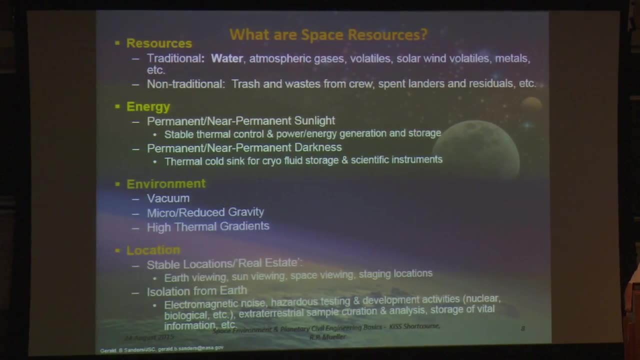 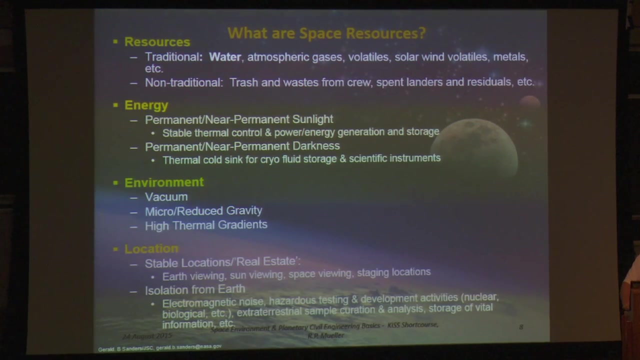 Might be a lot of metals or composite materials, carbon fiber, that you could repurpose, reuse, recycle, So that's non-traditional. Energy is also a resource. Permanent sunlight, non-permanent sunlight, darkness, The difference between sunlight and shadow. 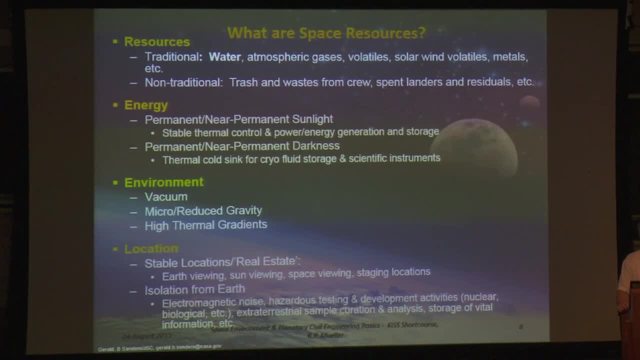 gives you a temperature differential which could potentially be harnessed to run, for example, a Stirling engine. So energy is- There's a lot of energy in space from the sun and we can harness that The environment. A lot of people don't think of a vacuum as being a positive thing. 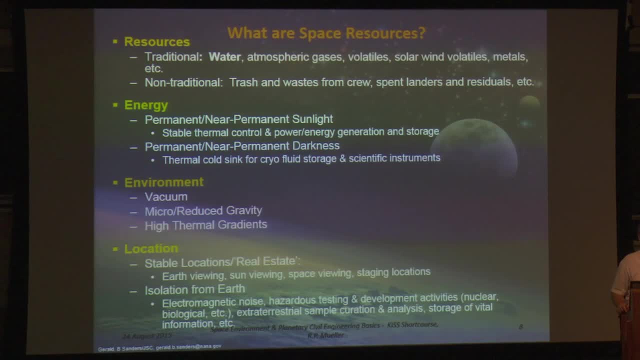 But if you're involved in manufacturing on Earth, a vacuum is a very useful thing, because now you can manufacture things in a pure vacuum. So sometimes the vacuum environment can help you. The micro-reduced gravity can also help you. We're doing ISS experiments to see how the microgravity 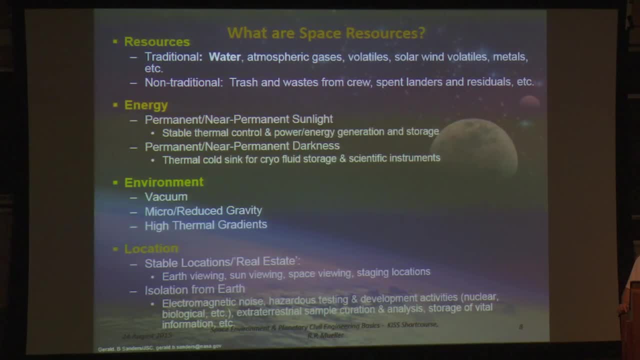 could actually help certain processes, things like growing crystals and other scientific phenomena. These high thermal gradients: they're bad, but they can also be harnessed if you think about it the right way. And finally, location, These liberation points: they're stable spots in the orbits. 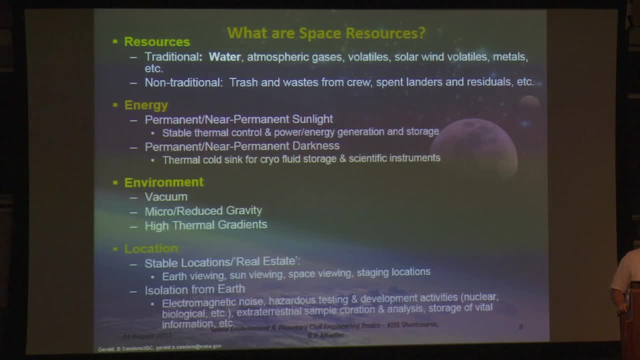 So if any two-body problem has these Lagrange points and so we can actually position spacecraft there and minimize the amount of propellant used for station keeping, And if you're on the far side of the moon, for example, you can be isolated from electromagnetic noise from Earth. 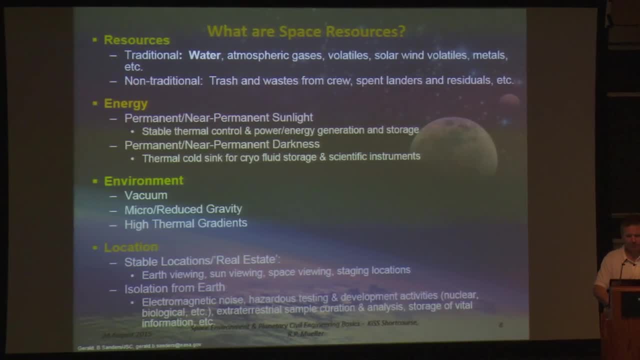 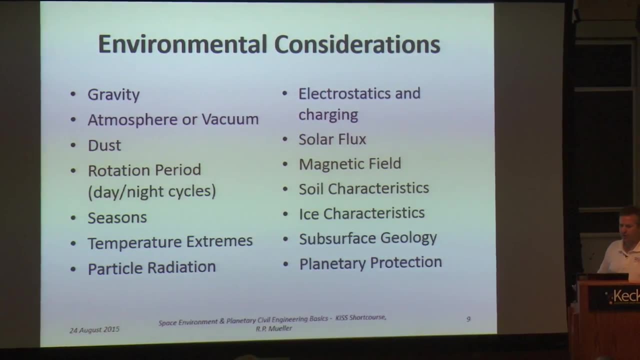 so that might be a good place to place a telescope, a radio telescope. So when we're on another planet, we have to think about the environmental considerations. and I won't go through all these in the interest of time, but here's a list of all the different things. 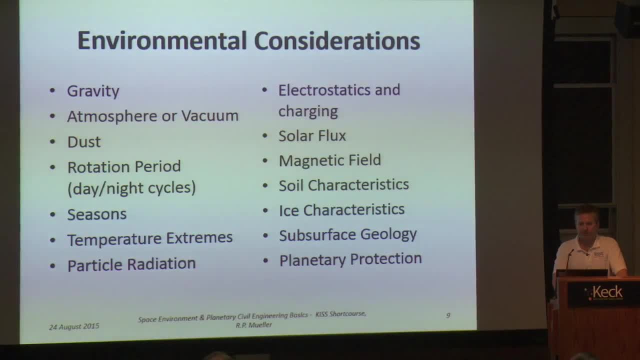 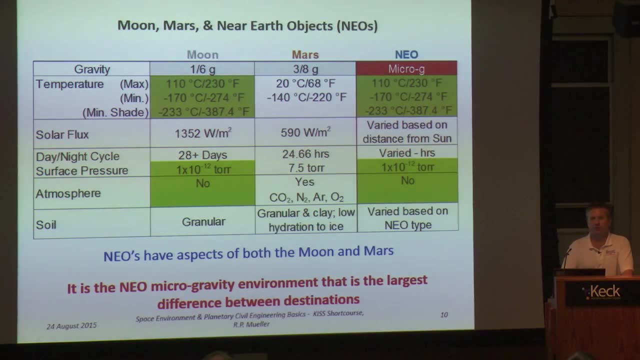 that need to be considered in terms of environment, Focusing just on these three locations: Moon, Mars and NEOs- near-Earth objects- so that could be an asteroid or a comet- and just look at these, Look at these temperatures. 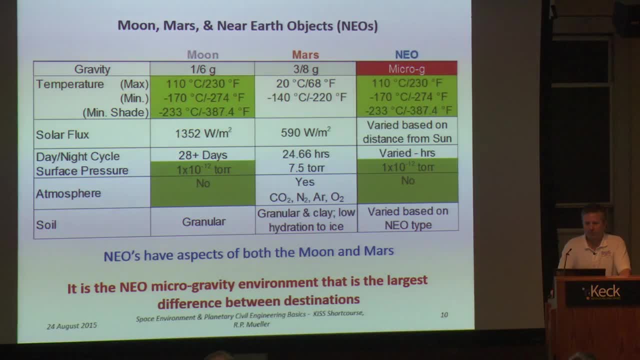 There's a wide temperature swing and fairly low temperatures. The Moon minus 170 C. In the shadows it's 40 Kelvin in the permanently shaded area, so it's minus 233 C. NEOs are also very cold and the Moon at the equator can get very hot during the daytime. 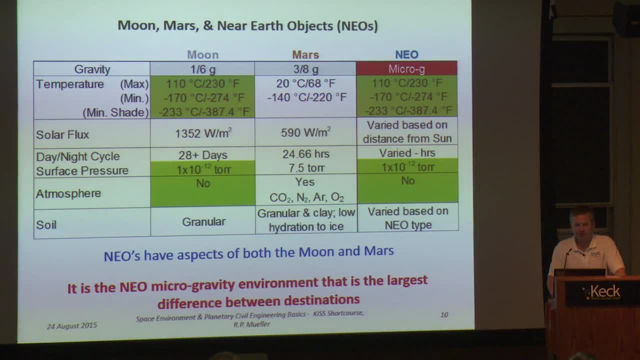 110 or higher Solar flux is very good on the Moon. It's a little bit further away from the Sun so it gets lower, but it's still a resource. Day-night cycle On Mars and NEOs this is not such a big consideration. 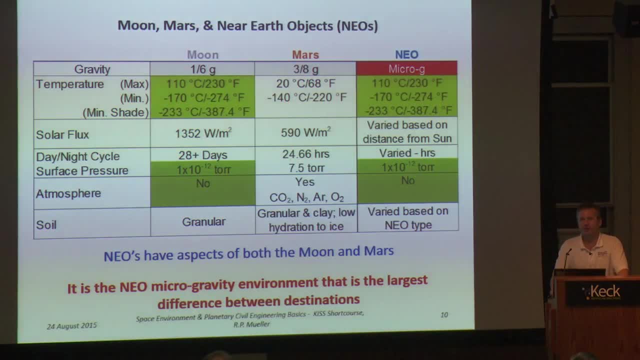 but surviving the lunar night is 14 days of lunar night and that's a big challenge right now. Nobody's ever done that yet. No atmosphere on the Moon. There is an atmosphere on Mars, which is considered a resource, and the soil, the regolith, is a resource. 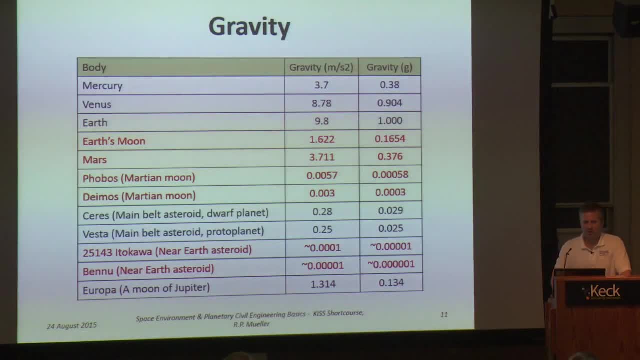 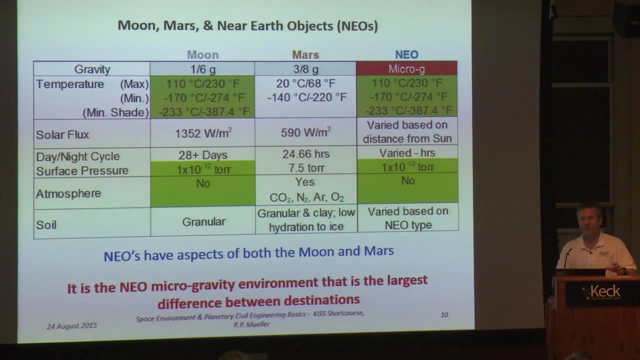 Almost everything we need is in the regolith. Let's just go back. The biggest difference between these three destinations is the microgravity environment on an asteroid or an Earth object. That's really the dividing line. Partial gravity is one type of environment. 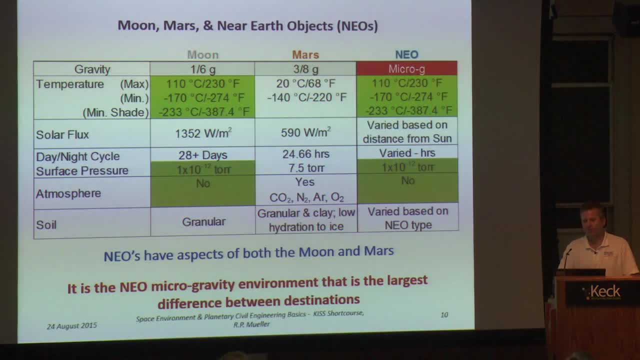 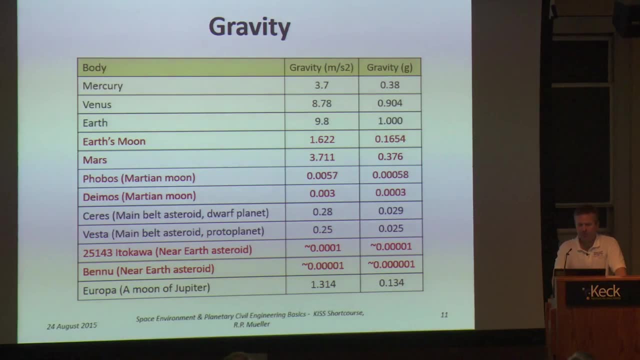 and reduced gravity. microgravity, milligravity is another environment and I would say those are two distinct environments And that's what we're showing here. One thing that is interesting which caught my attention recently was the gravity on Europa is about the same as the gravity on Earth's Moon. 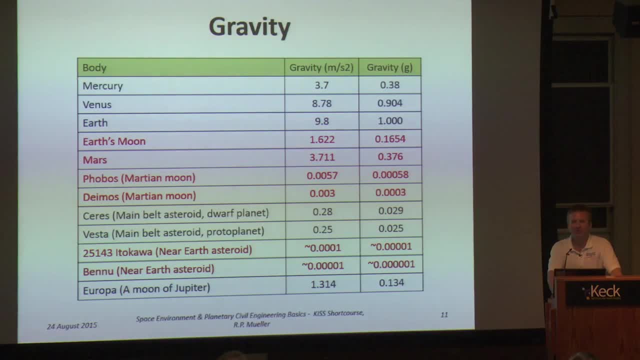 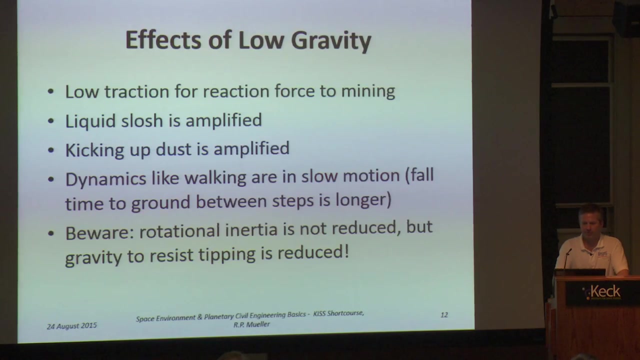 so that's a little piece of trivia for you. You might win a prize on a trivia contest if you know that one. So you can see, the gravity is mostly less than on Earth, and so we have to deal with reduced gravity phenomena. So what does that mean to us? 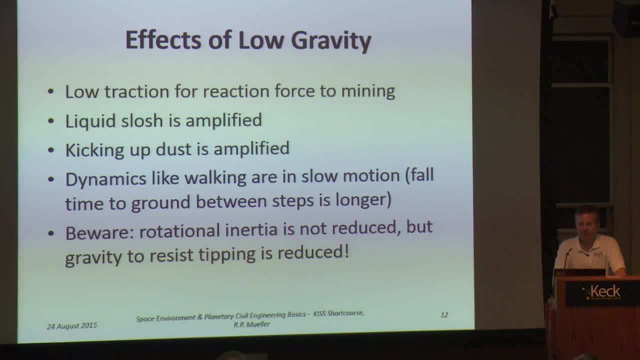 What are the effects of low gravity? Well, first of all, if you tried to dig in a place like the Moon and you had a traditional front-end loader and you tried to push in, depending on the size of the machine, 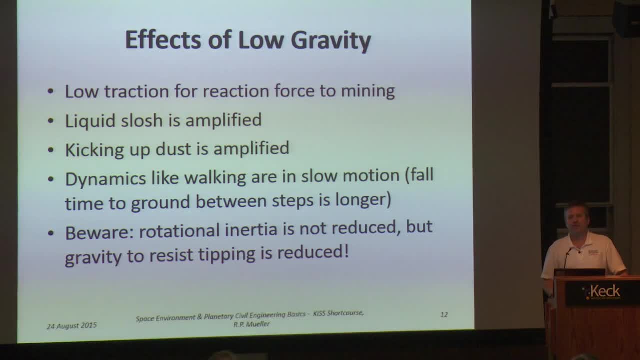 but let's say it's a small machine, because we can't launch these giant yellow heavy equipment machines into space. they're just too heavy. So we probably have small machines. If you had a small front-end loader it would try to dig. 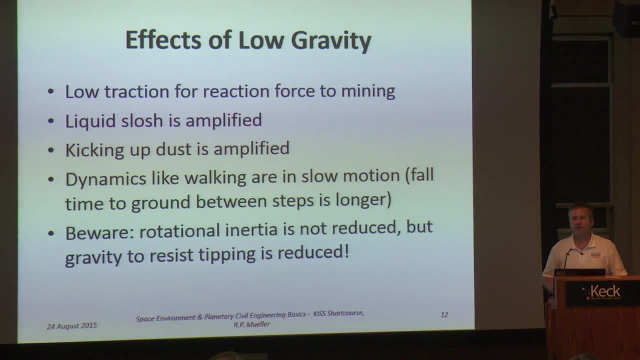 and it wouldn't actually have enough reaction force due to its own weight to penetrate the soil. It would do a push-up. It would not penetrate the regolith. So we have to find new ways of digging and that's what we're working on. 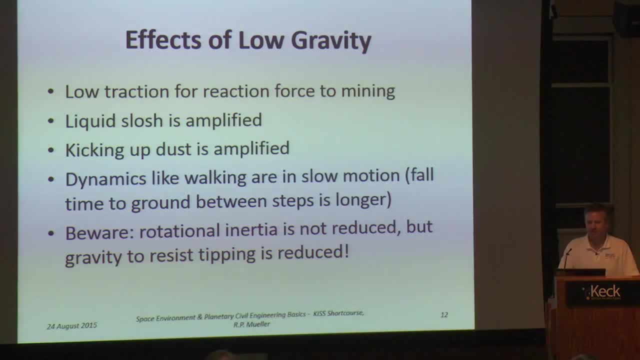 Liquid slosh is amplified, Kicking up dust is amplified, Dynamics like walking or slow motion. if you remember, in the Apollo missions the astronauts were doing kangaroo hops. They were hopping not because they were playing around, but because that was a more efficient form of locomotion. 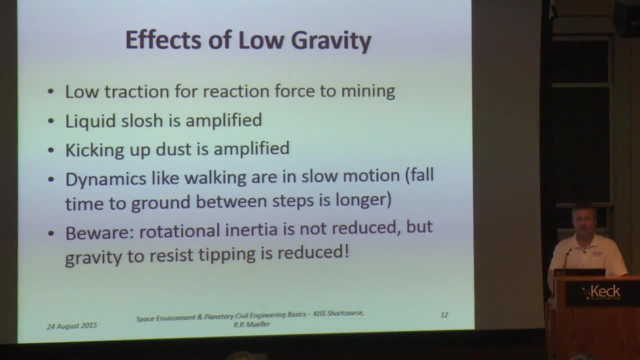 So there's different solutions out there, And be careful, because in a low gravity environment you will have the inertia forces will not be reduced, And so if you had a mass, say a boom on a crane and you swung it to the side. 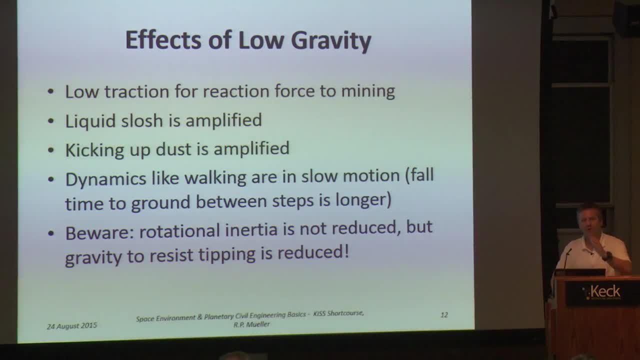 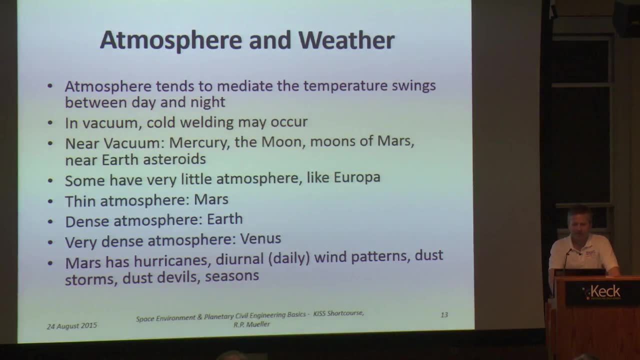 it would still have the same inertia but less gravity, so it might tip over on you. So these are all the practical considerations. The atmosphere is very important because the atmosphere is a way of mediating the temperature swings. It's a buffer. 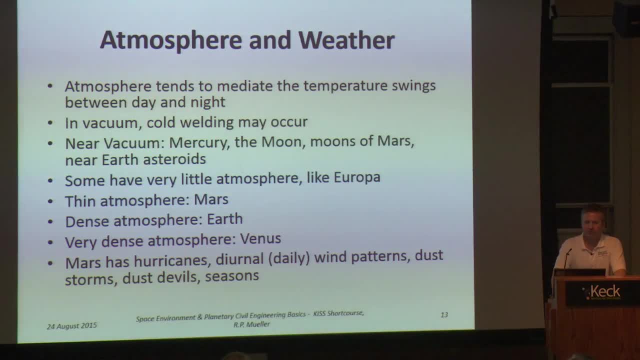 and it keeps things temperate. But when there is no atmosphere then you have larger temperature swings. In a vacuum culture, cold welding may occur. This actually happened in some space missions where the hatch of the capsule- I believe it was in the Mercury missions- 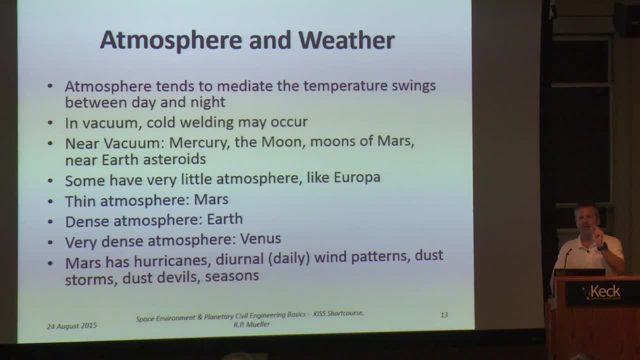 or some of the early missions. the capsule had a hatch, actually cold welded, shut in a vacuum. So these are things, practical considerations you have to think about. Some places have very little atmosphere: The asteroids. Mars has a very thin atmosphere. Earth has a dense atmosphere. 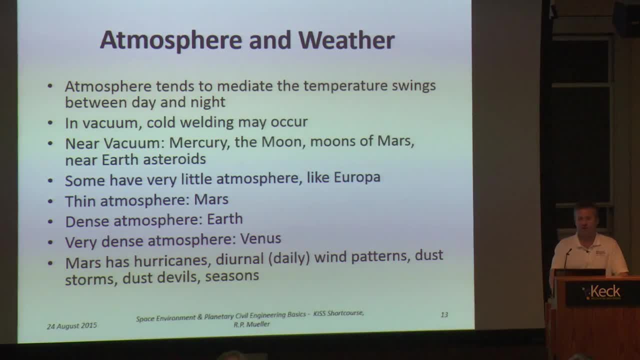 Venus has a very dense atmosphere. Mars has weather, has hurricanes, has earthquakes, has wind patterns, dust, storms, dust devils, seasons- These are all things that have to be considered. If you were building a house, you'd want to build it in a place that had good weather. 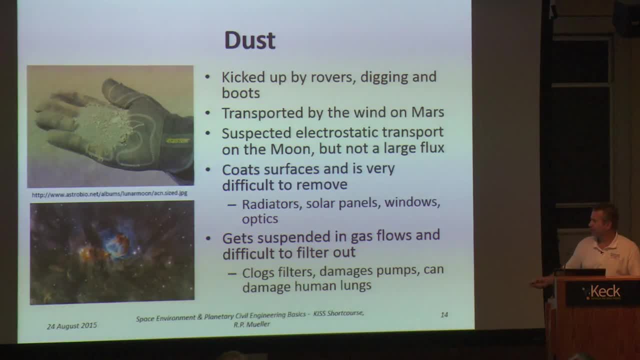 Dust. dust is everywhere. The whole universe is full of dust and all planetary surfaces are covered in dust, and to varying degrees, And this instead of thinking negatively about this. this dust or regolith, it's a resource. However, you also have to deal with it. 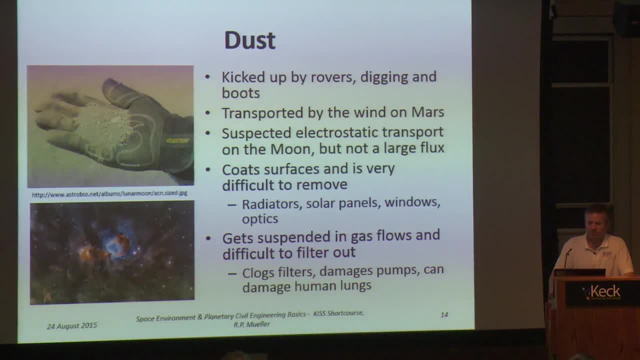 It's transported by the wind on Mars, it's kicked up by rovers, it's on the moon, it gets electrostatically charged from the sunlight And so it's highly electrostatically charged and the solar terminator passes by, possibly levitates it. 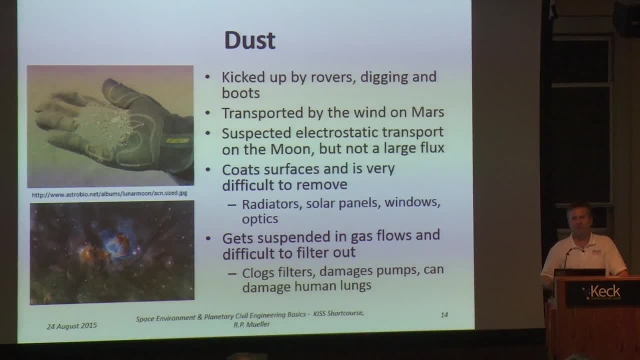 it's not known yet. and it coats surfaces, And because these particles are under 100 microns, the van der Waals forces also dominate. So you have electrostatics, you have van der Waals, you have these very, you have these very convoluted morphologies of each particle. 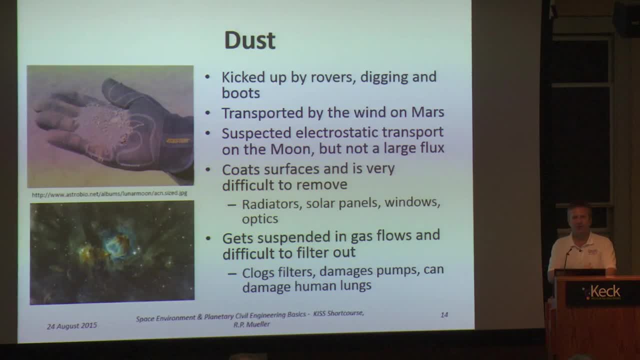 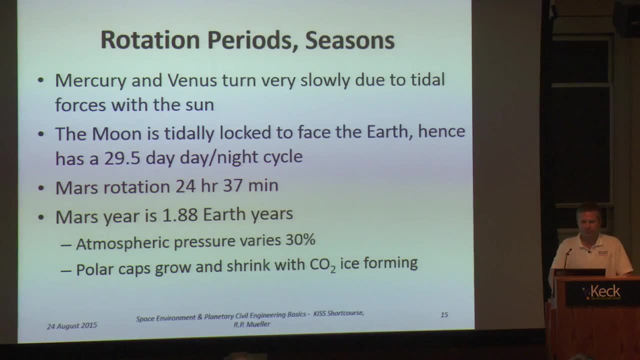 creates a lot of friction. So in the Apollo missions the suits were covered with dust. it was very difficult to get them out. It also clogs filters, So it's a big challenge. The seasons: every destination has a different type of rotation period. 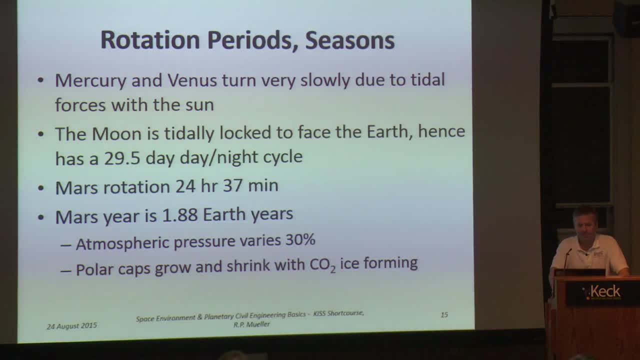 and different seasons as a result of its orbit. So the moon is tidally locked with the Earth, 29.5 day-night cycle, so slightly longer than 14 days: Earth days for a moon day and 14 Earth days for a moon night. 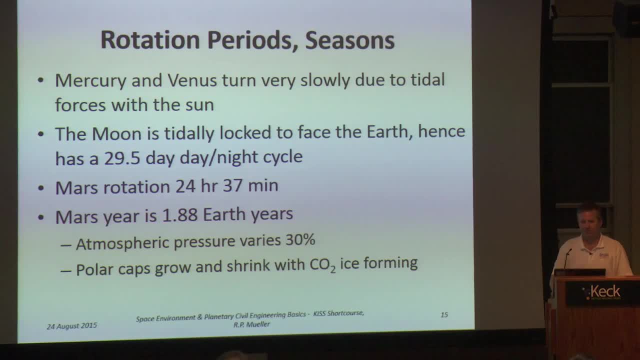 Mars rotation is slightly longer than the Earth day- 24 hours and 37 minutes, which is not too bad. A Mars year is 1.88 Earth years. The atmospheric pressure on Mars varies by 30%. The polar caps grow and shrink. 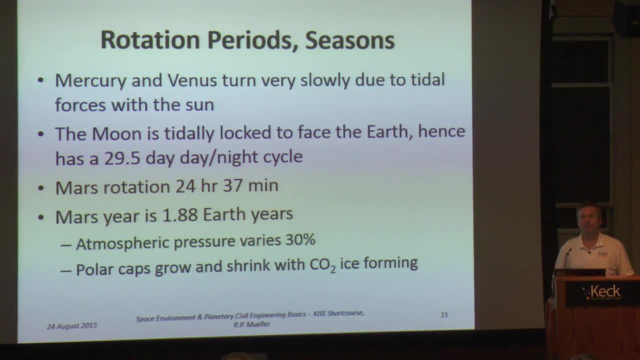 and actually there's meters of CO2 ice form at the Mars poles in the winter. So if you were building a habitat at the Mars poles and in the winter you were covered with meters of CO2 ice, that might be a consideration. Could be useful too. So the temperatures is something we have to consider. The moon has high temperature swings: minus 173 degrees to plus 117.. Polar crater is 40 Kelvin. Mars is not as bad as the moon: minus 125 to plus 20.. 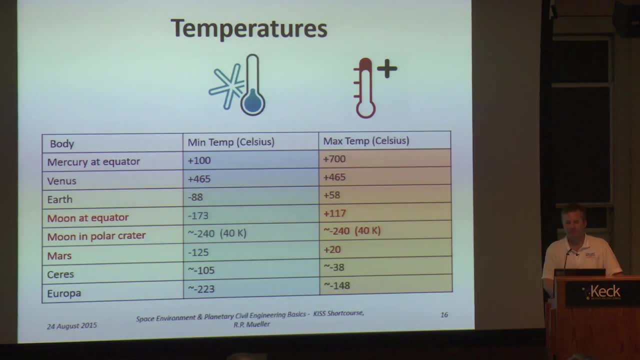 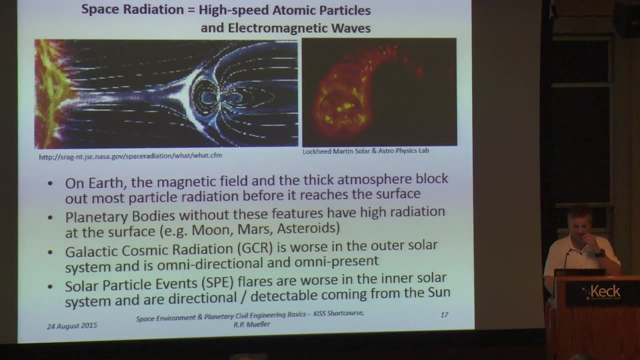 There are regions on Mars that are actually quite reasonable, So that's why it's been considered friendly for human habitation. Space radiation is a big problem. We have high-speed atomic particles and electromagnetic waves. There's basically two types of space radiation. There's galactic cosmic radiation. it's worse than the outer solar system. it's background radiation from the universe and it's omnidirectional and omnipresent. Solar particle events originate from the sun and they're event-driven, So they're not always there. 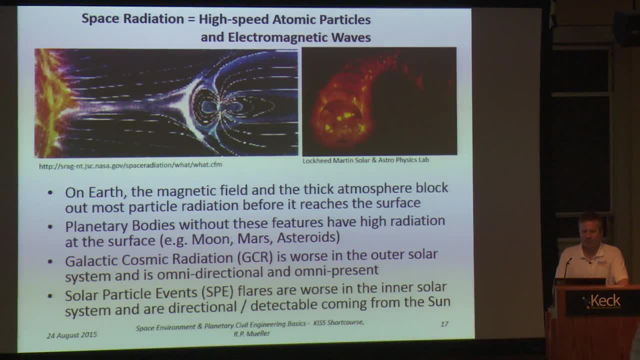 but they periodically flare up. It's a cycle And they are detectable. So a lot of times I talk about space weather prediction, So some kind of a warning system that would let you duck into a shelter. So that's another consideration. 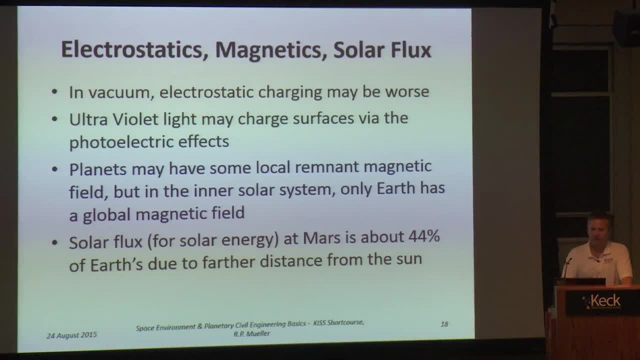 is, should we build a shelter? We already talked a little bit about electrostatic charging. The ultraviolet light may charge surfaces via photoelectric effects and some planets have local remnant magnetic fields, But in the inner solar system only the Earth has a global magnetic field. 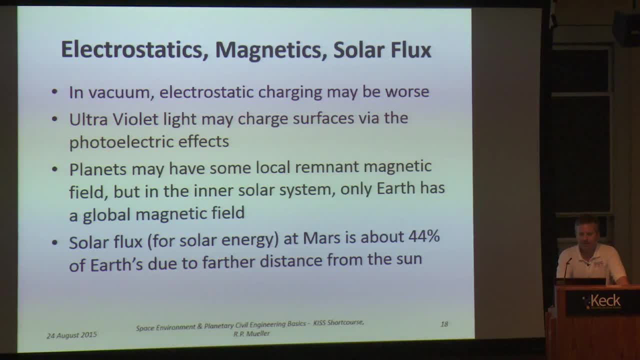 due to its liquid iron core, And so you cannot rely on, for example, a compass when you're navigating on another planet, and certainly not GPS Solar flux at Mars- about 44% of Earth's- due to the further distance from the sun. 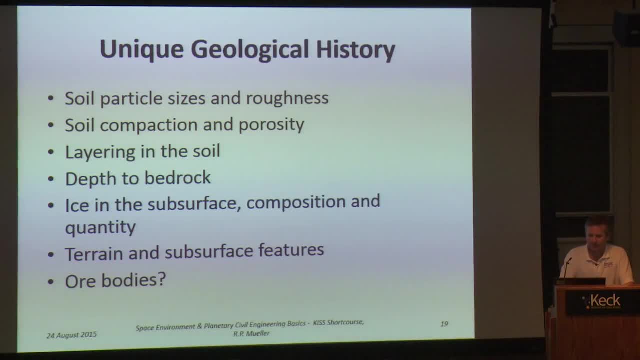 and they have dust storms too, which attenuates the light. Soil particles, size and roughness, soil compaction, porosity, layering of soil depth to bedrock ice in the subsurface terrain, subsurface features- these are different. 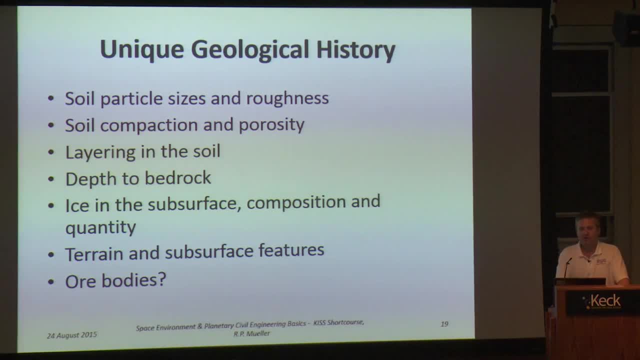 Every destination you go to is different because they all form differently, And so what we're interested in in ISRU- in-situ resource utilization- are the ore bodies. An ore is defined as a useful substance. An ore has to be economically viable. 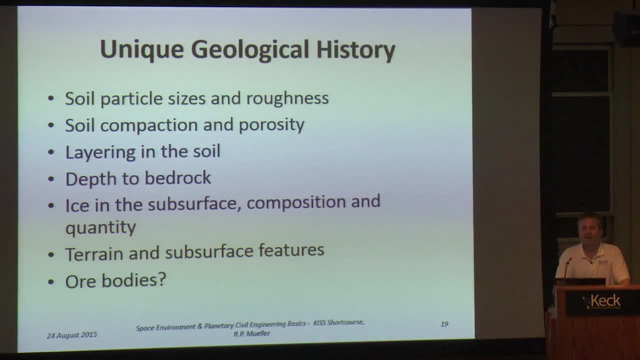 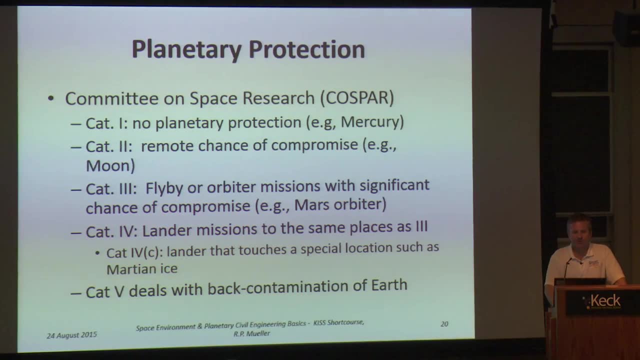 If you mine something and it's not economically viable, it's not an ore. One thing that we have to consider as a human species is planetary protection. So there's a committee on space research and their job is to make sure that. 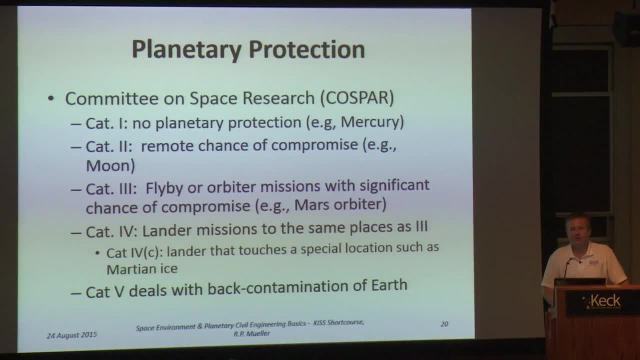 no harm falls on the human race, either by forward contamination or backwards contamination, And so we have to be very careful that we don't contaminate the destinations that we go to or that we bring something back from Earth that could wipe out the human species. 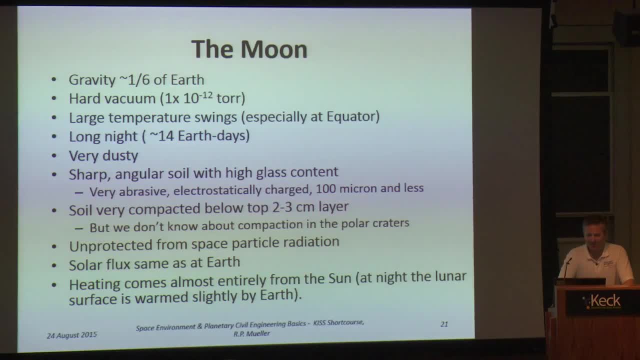 Kind of important Moon, one-sixth of Earth: hard vacuum, large temperature swings, long night, very dusty, sharp angular soil with high glass content. it's very fluffy. they call this- this is a real scientific term- fluffy regolith. 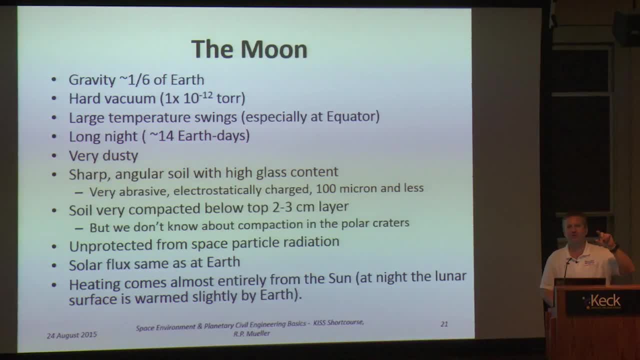 The top two to three centimeters of the moon are fluffy and that's very loose, low average density. but then it rapidly compacts Within about 30 centimeters. it's highly compacted. It's unprotected from the moon is unprotected. 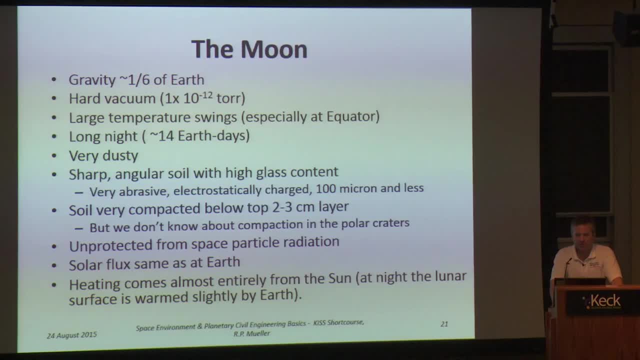 it has its own. it has no atmosphere, no magnetosphere and the solar flux is the same as on Earth. but it's a very radiation heat transfer dependent phenomenon. It comes most of the heating comes from the sun, Near Earth, asteroids. 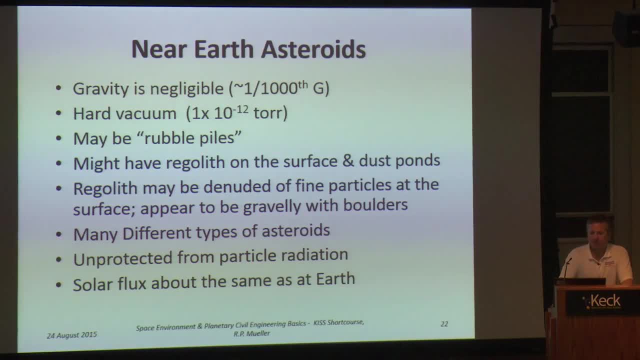 one-one-thousandth G, so milli G. hard vacuum, maybe rubble piles. So the cartoon version of an asteroid is this metallic object floating in space. Well, some are like that, but most are not. Most are rubble piles. And the rubble piles are loosely held, dust and rocks floating in space, held together by electrostatic forces, van der Waals forces and some gravity. So change your mindset. An asteroid is not a chunk of metal floating in space. It's a collection of loose debris. 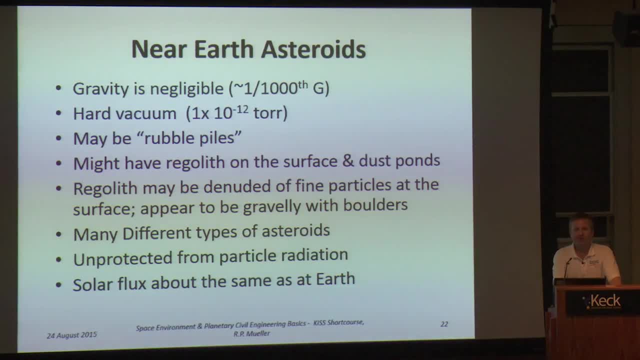 There might have, might be, regolith on the surface. This is not fully understood yet, but we have seen dust ponds- dust ponds on asteroids, so that's very interesting, And it appears that the solar wind blows the fine particles off and they're gravelly with boulders on the surface. 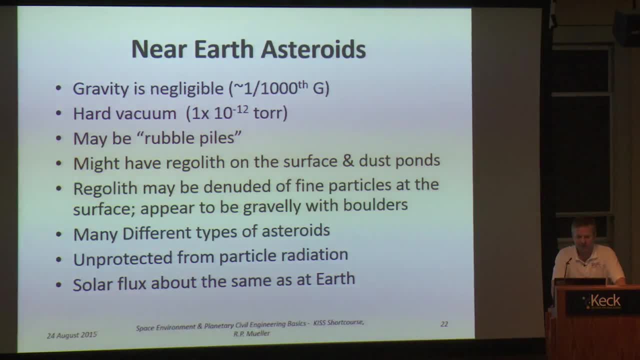 but the dust might be below the surface, We're not sure yet- Many different types of asteroid. It's unprotected from particle radiation and the solar flux is about the same as on Earth. Mars- well, we have a lot of Mars experts at JPL and Caltech. 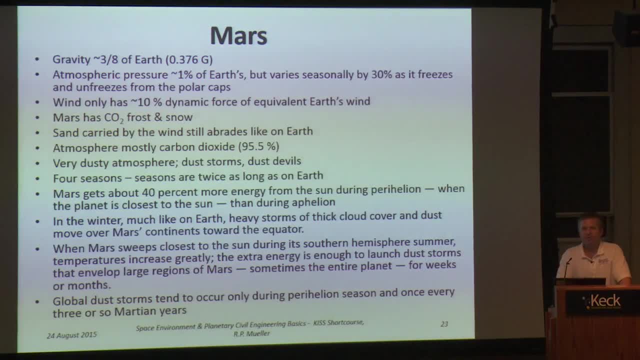 We're much more familiar with Mars, much smarter about Mars than we were even ten years ago. A very interesting place. Three-eighths the gravity of Earth. The atmospheric pressure is 1% of Earth. so there is an atmosphere, but it's barely an atmosphere. 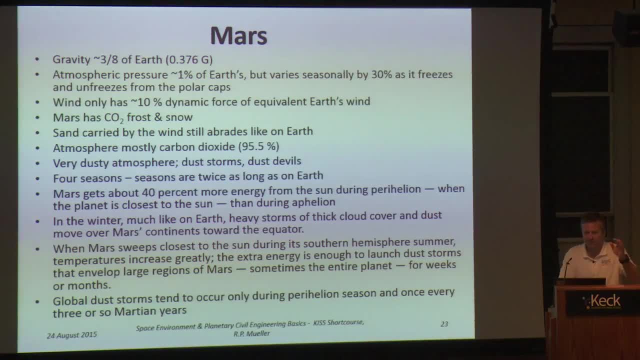 95.5% CO2 varies seasonally by 30% as it freezes and unfreezes from the polar caps. If you're standing on the surface of Mars and there's a 100-mile-per-hour wind, it actually the dynamic force. 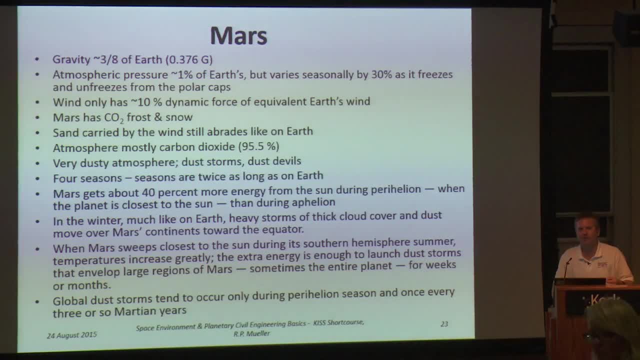 will be 10%, so it'll feel like a 10-mile-per-hour wind. So even though people talk about hurricanes on Mars, it's not exactly the same because the dynamic pressure is lower. So it's about 10%. Mars has CO2, frost and snow. 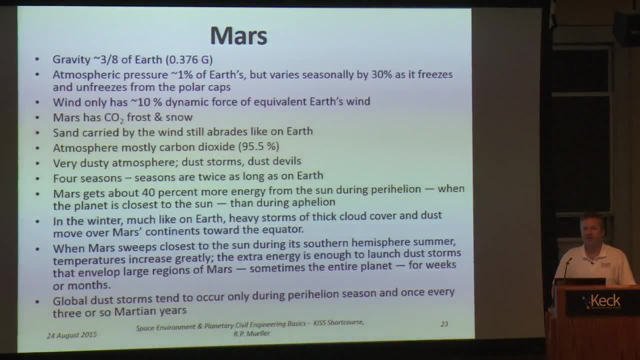 We've seen that. We've seen pictures of CO2.. Even Viking had it- of CO2, frost and even snow coming down in the sky on Mars. Very interesting: Sand is carried by the wind and it abrades like on Earth. 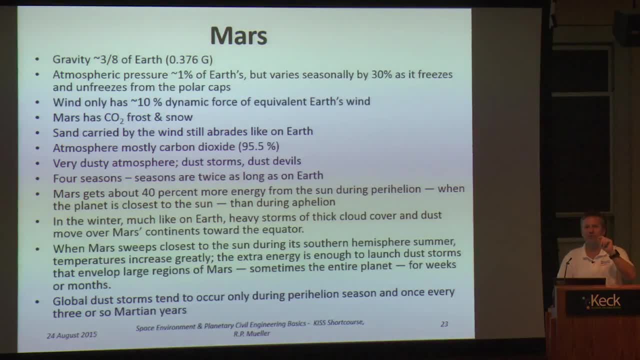 So the particles on Mars are not sharp like on the Moon. They're rounded more like beach sand because they've had weathering. I've already said the atmosphere is mostly carbon dioxide. It's very dusty, dust, storms, dust devils. These dust devils they cleaned off the MER solar panels. 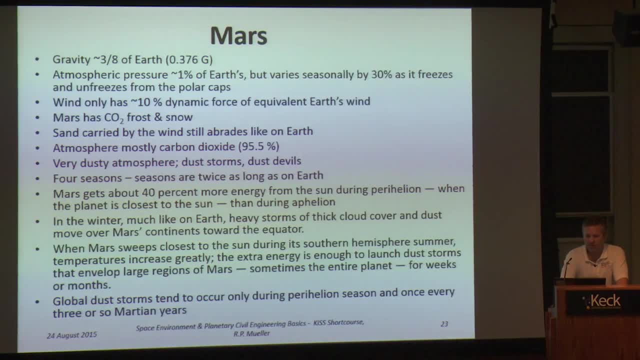 so we have proof of that. We have seasons. The seasons are twice as long on Earth. Mars gets 40% more energy from the Sun during perihelion, when the planet is closest to the Sun, than during aphelion. So that affects the seasons and the weather. In the winter, like on Earth, you have heavy storms of thick cloud cover and dust that move over the Mars continents towards the equator, And then, when it's closer to the Sun, then the temperatures increase quite a bit. 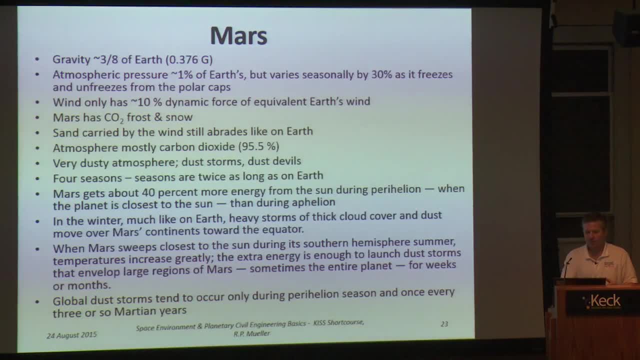 and you have extra energy. So then you have large dust storms. Sometimes these dust storms last for weeks or months and cover the entire planet. So it's something we'll have to deal with, And global dust storms tend to occur only during perihelion season. 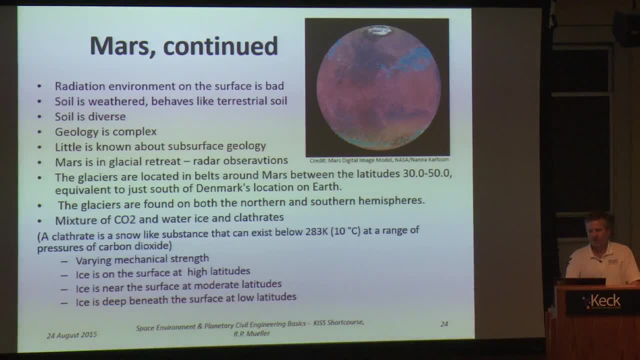 once every three or so Martian years. So that's it. So we know so much about Mars. I have a second chart about it. The radiation environment on the surface is bad, Soil is weathered, Soil is diverse, The geology is complex. 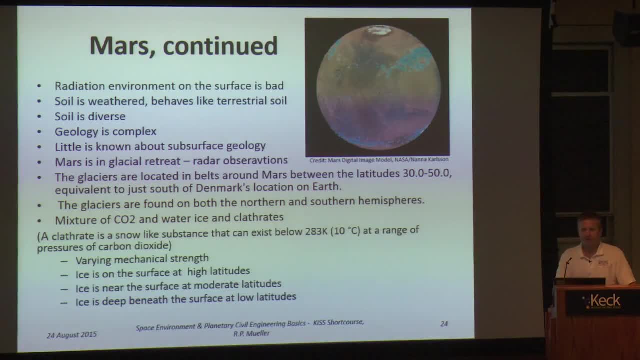 Little is known about the subsurface geology. Some people believe Mars is in glacial retreat. based on recent radar observations- The picture you see on there, those little blue dots- are suspected to be subsurface glaciers that are kept from subliming. 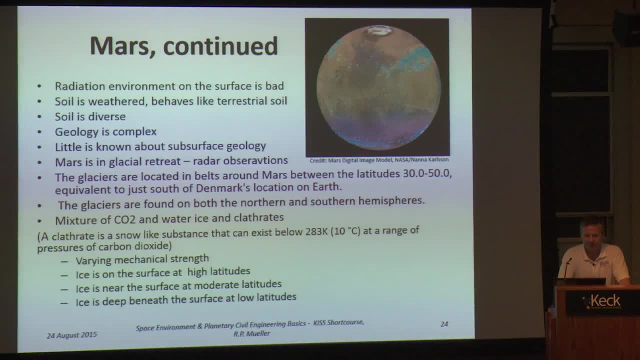 by the regolith that creates an insulating layer. So between 30 and 50 degrees north and south latitude. that's where we suspect some of these glaciers might be found And we have a workshop that we'll have in October to discuss these locations on Mars. 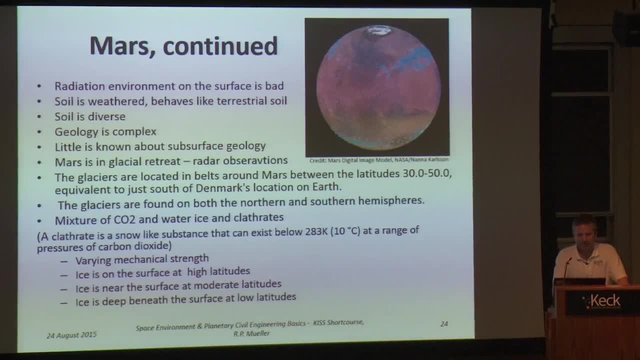 and what would be best for landing humans. There's a mixture of CO2 and water, ice and clathrates. It's a snow-like substance made of carbon dioxide, And so there is ice on Mars, but we have to find it. So, in summary, on the environments, 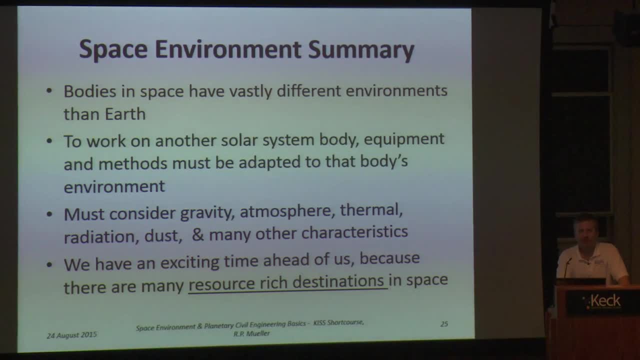 we have vastly different environments than on Earth And that affects the way we solve our problems. We'll have different solutions based on the different environments. We have to adapt. We have to adapt to those other environments And, like I said, it's maybe a change of mindset. 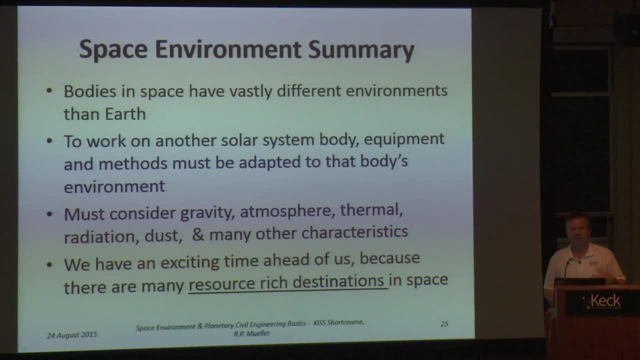 Instead of thinking of everything as a problem, think of it as an opportunity. A vacuum is an opportunity. A large temperature differential is an opportunity. There are things we can do if we change the way we think. So that's what we have to do. 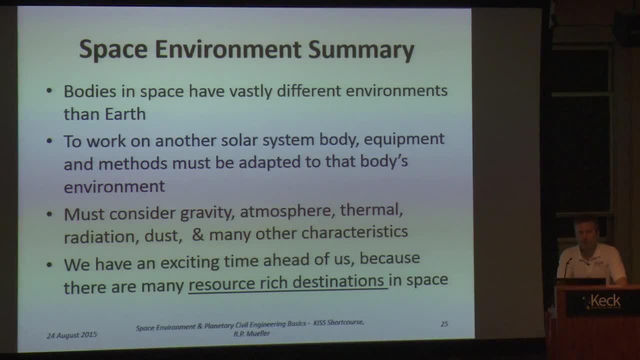 We have to consider gravity when we're designing structures in space- civil engineering structures. Then we have to consider gravity, atmosphere, thermal radiation, dust, many other characteristics. Overall, we have a very exciting time ahead of us because there are vast amounts of resources in space. 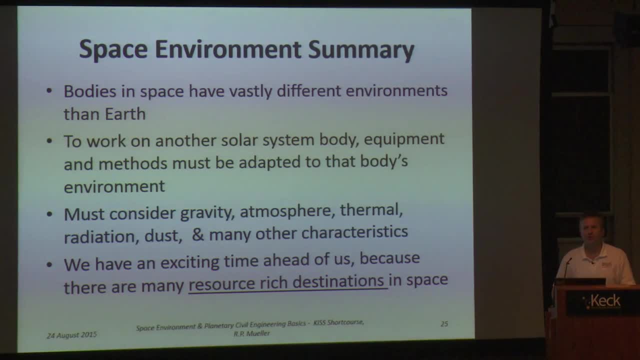 If we can learn how to harness those resources, we will not be resource or energy constrained. Now there's a price to pay for that. We have to learn how to use these resources, We have to develop the technology, We have to make an investment to harness these resources. 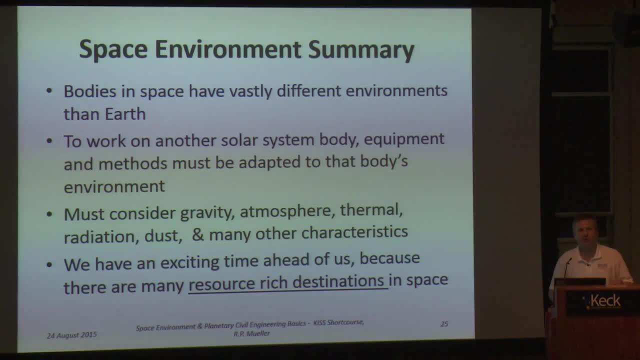 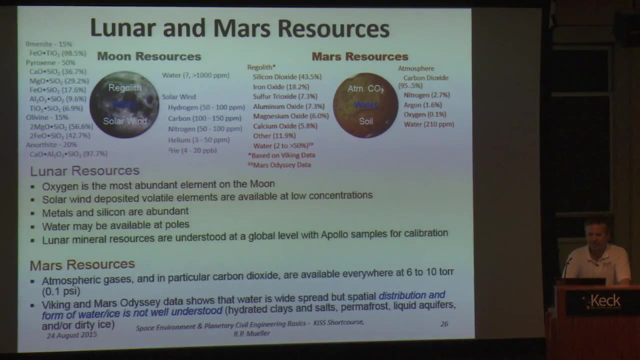 But they are out there, So all we have to do is figure out how to harness the resources. I'm not going to go into this in detail in the interest of time, but this is a list of all the minerals, And most of these minerals are very useful. 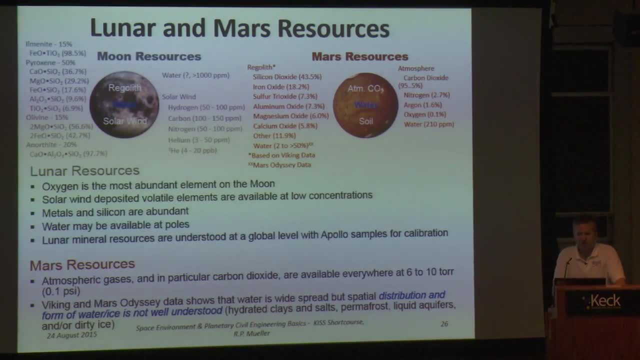 But you'll see there's a lot of oxides. So oxygen is the most abundant element on the moon. 42% by mass of the regolith on the moon is oxygen. You scoop up a kilogram of oxygen, you can get 42% of regolith. sorry. 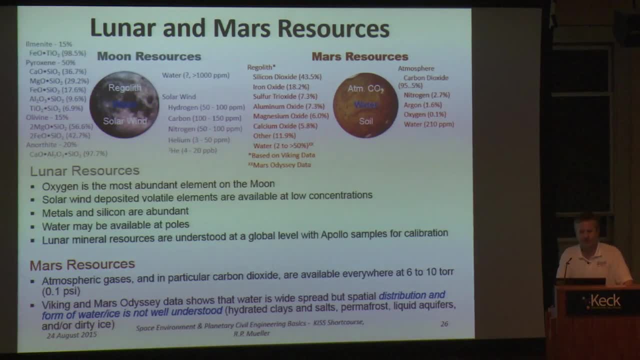 you can get 42% by mass of oxygen out of that. Metals and silicon are abundant. Water may be available to poles. Mars atmosphere is a resource. You can extract oxygen from the Mars atmosphere And we've shown that water is available either as water, ice or as hydrated minerals. 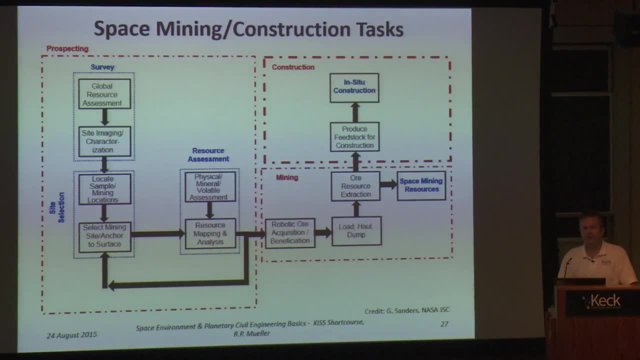 Now let's get into more of the. we understand the environment. now We've been through the environment And we'll get into the engineering side, And this is basically the flow, the engineering flow of space mining instruction, And they're mutually beneficial. 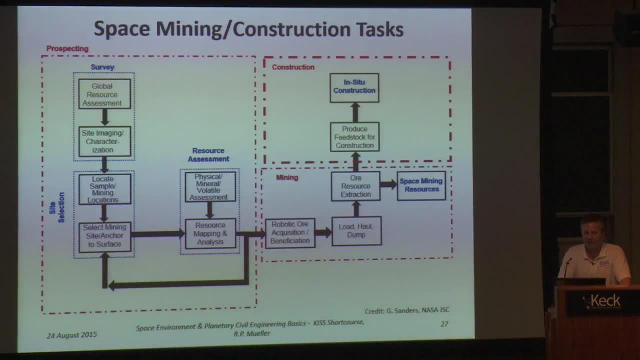 Because the first step of space mining is to find the resources. Once you've found the resources, you characterize the resources, then you acquire the resources, Then you extract the ore And then you have a waste material. Well, it turns out that after you've extracted, 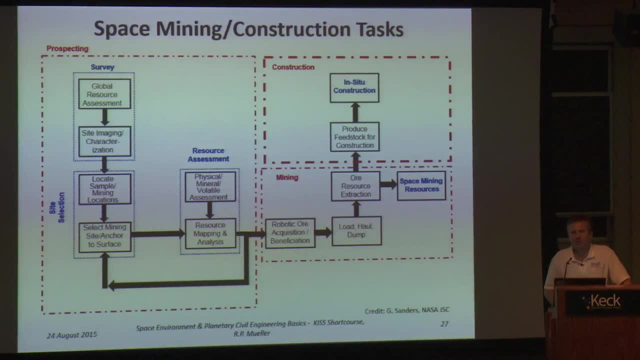 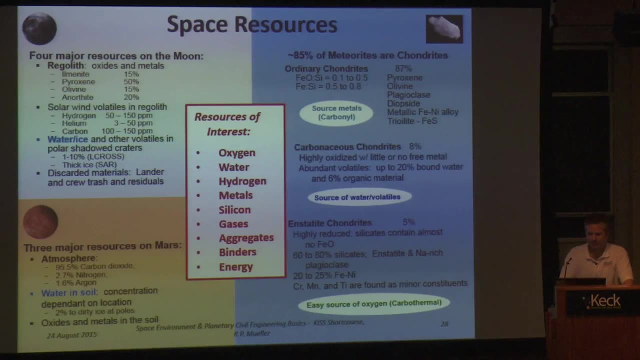 your useful ore from the material. the waste material can be used as an aggregate for civil engineering material, So it's all complementary and synergistic. The resources of interest in space that we're looking for are oxygen, water, hydrogen metals, silicon gases. 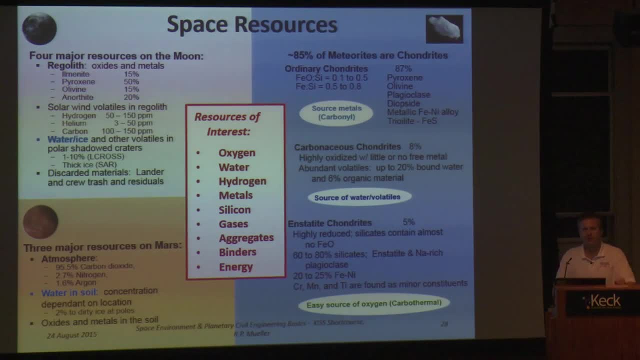 Then for civil engineering. this is kind of new. Most scientists haven't thought in these terms recently. Aggregates, binders and energy to do something useful with these materials. A few years ago we looked at this whole trade space. 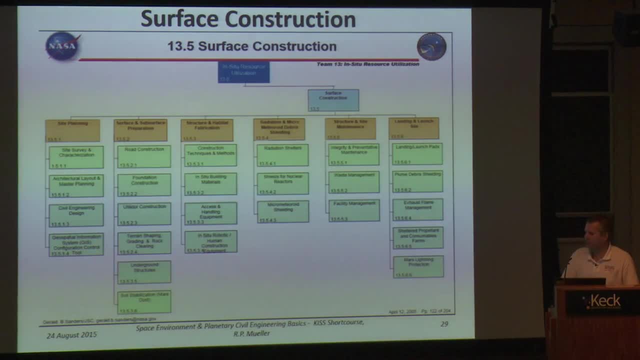 And we said: what is surface construction? This was part of a NASA road mapping activity. What is surface construction? Well, it's similar to surface construction on Earth, but the solutions will probably be different. So we basically have a a work breakdown structure here. 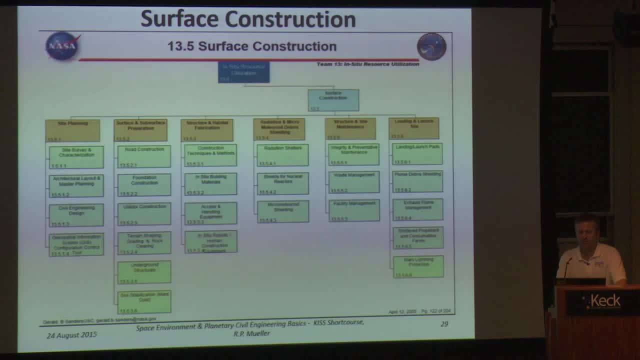 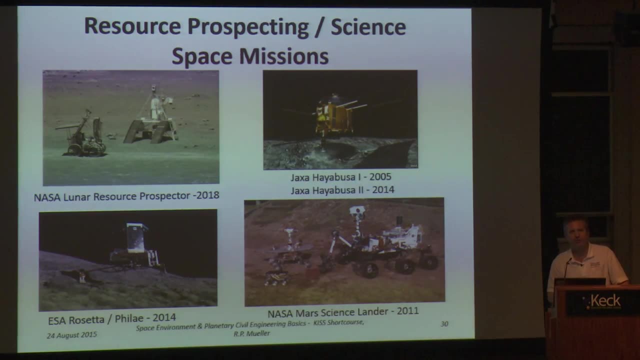 of all the different tasks that we'd have to go do in space to do surface construction. Now, today, this is what a typical space mission looks like, And we're in the prospecting phase. So everything you see today is in the prospecting phase. 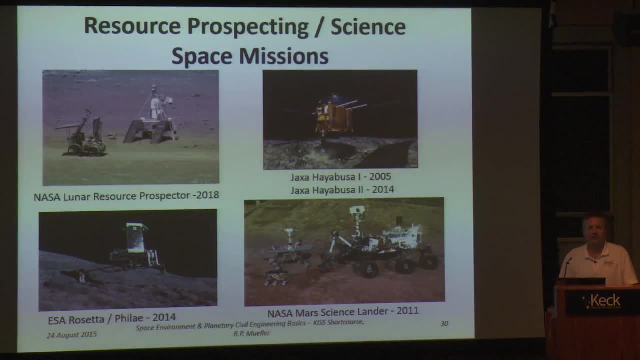 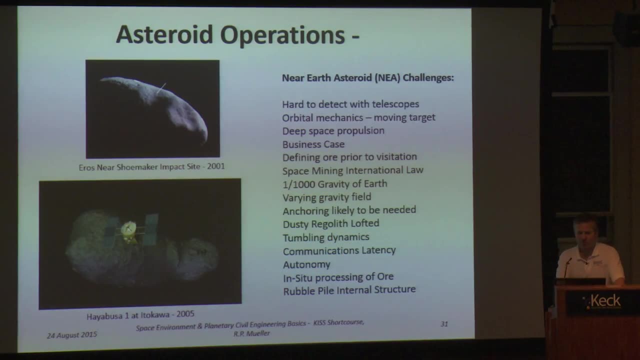 It's being done for science reasons and in some cases for resource prospecting goals On an asteroid. we have some really unique challenges And we'll discuss those later in the workshop. But it's hard to detect. These asteroids are hard to find. They're small objects in the vastness of space on a dark background, So they're hard to detect with telescopes, Orbital mechanics. they're moving targets, So you have to understand that It requires deep space propulsion. It's a long journey. 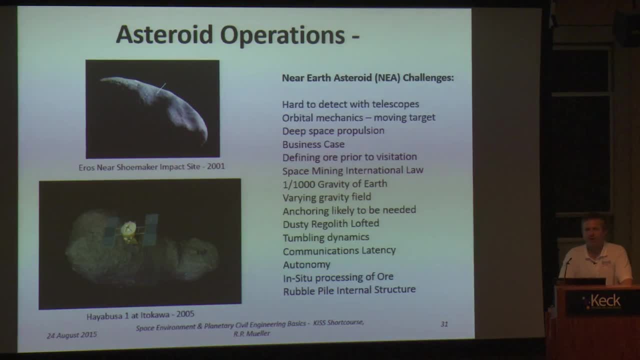 There has to be a business case. Is it cheaper to mine it on Earth or is it cheaper to go get it from an asteroid? It's as simple as that: Defining ore prior to visitation. We might go there and find there's plenty of ore. 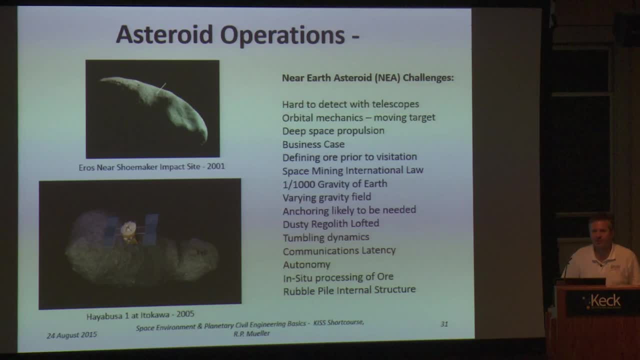 Maybe the mass spectrometer told us there was ore, but it's inaccessible. Could be a problem. Space mining international law: We have to understand the laws. Make sure that everybody's clear on ownership rights. No business will invest in a venture unless they have a legal right to do that. 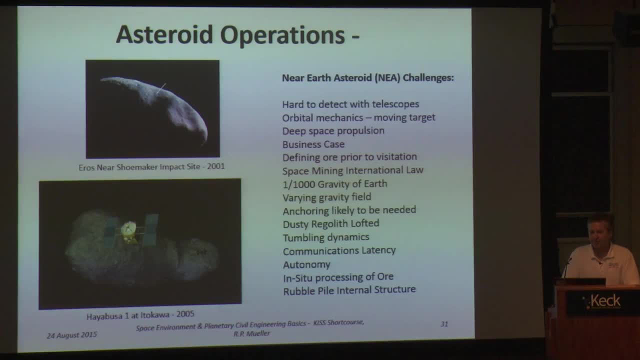 It's 1,000th gravity of Earth. It's a varying gravity field. Anchoring is likely to be needed. Dusty regolith will be lofted. If you have a thruster impinging on the surface of an asteroid. that cloud would last weeks. 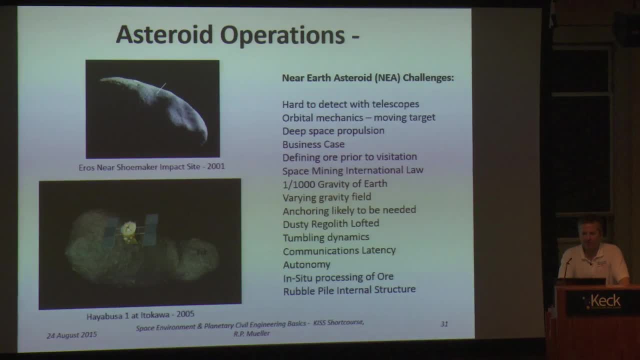 So you have to be careful. Tumbling dynamics: How do you synchronize with a tumbling asteroid Communications latency To Mars? in the worst case it's 20 to 40 minutes latency of communications each way. So you have to consider that. 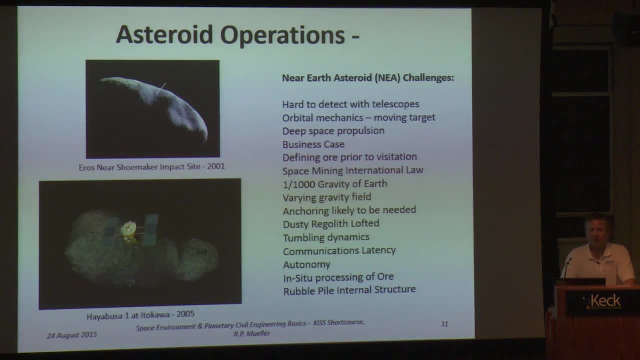 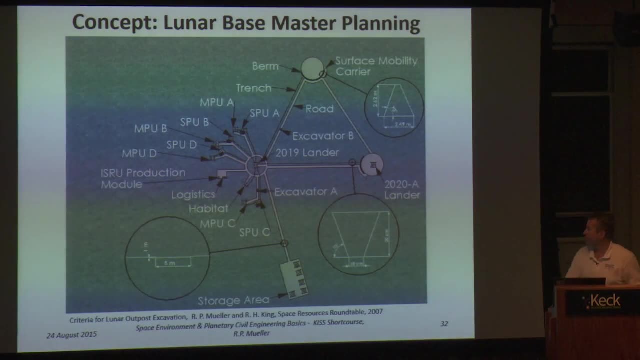 autonomy is likely to be needed. Do you bring the ore back or do you process it at the asteroid? And it's a rubble pile, most likely the internal structure, So that's asteroids. So if we were building a moon base a few years ago, we put together this notional concept. 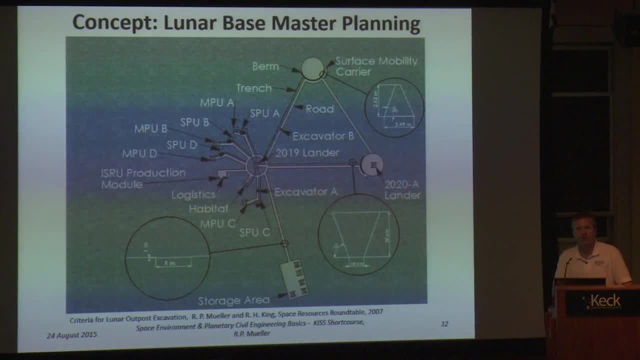 of a moon base, and I called it master planning. This is what civil engineers do. They do master planning of a community, or architects are very good at this too. So we have to do some master planning, And so it involves quite a few tasks. 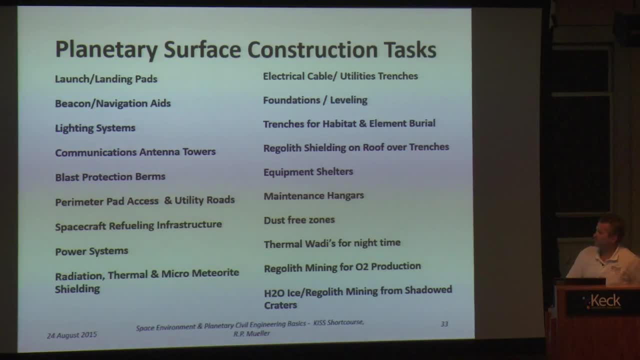 So what are the tasks? The planetary surface construction tasks? Well, this is a long list. People are always surprised. Well, it's not just landing, It's not just deploying a habitat. There are other things that need to be considered. 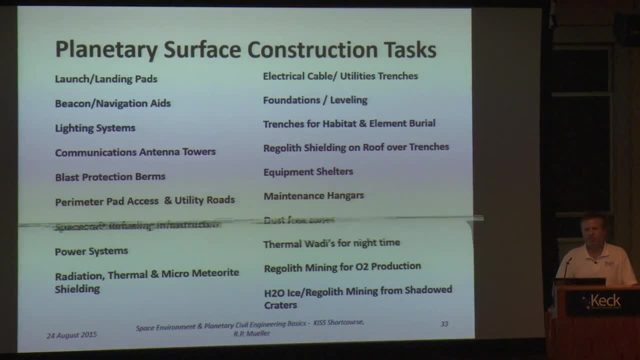 And here's a long list of them, And these are all what we call infrastructure, And, granted, that's a little bit further down the road when we're more established, but it is something to consider. What's very interesting is in the Constellation Program days. 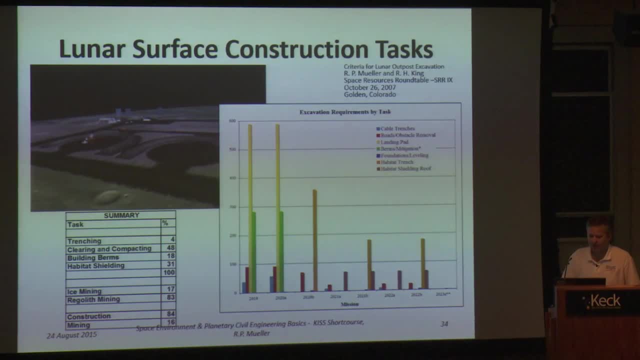 we did a study on how much regolith you have to excavate And maybe a surprising result is in the bottom right-hand corner Of all the regolith. this is just a bar chart. This is tons of regolith and this is the mission it was going to fly on. 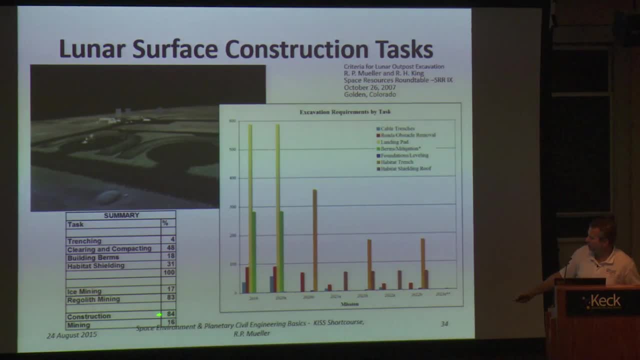 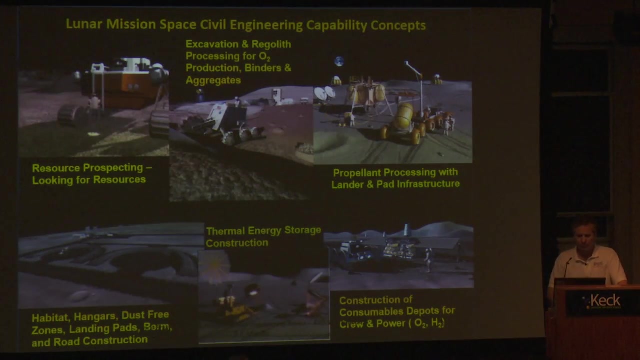 And of all that regolith, 84% was for construction by mass, 16% was for mining for extracting oxygen. So it was kind of an eye-opener that most of the regolith that needs to be excavated is for construction. 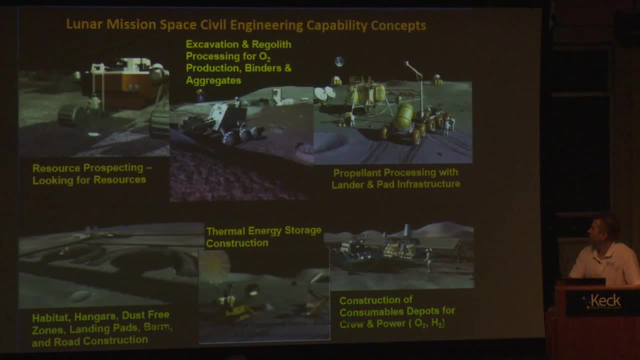 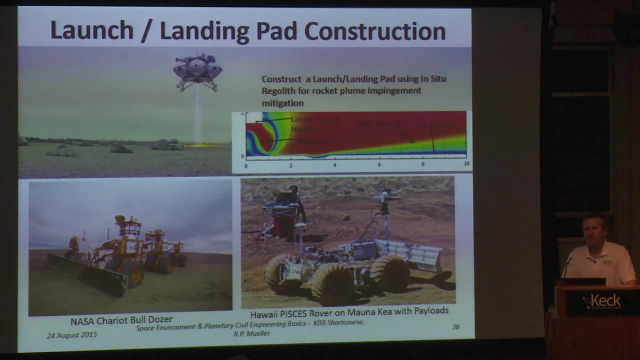 These are some concepts of what you could go do and what the artistic concepts, And so you can see there's plenty to do. Probably the very first thing we need to do is build a launch landing pad, in my opinion, because why would you risk landing repeatedly on an unstable surface? 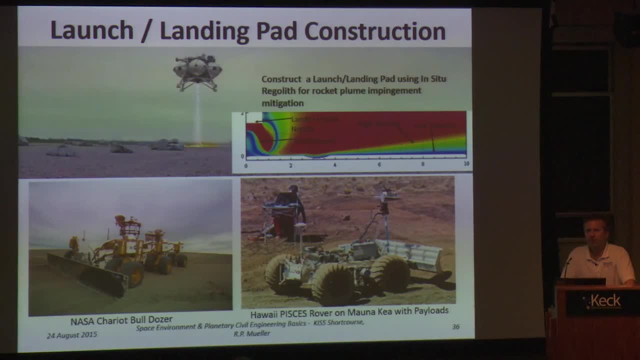 The risk is in the life cycle cost. One of the companies we're working with, Massen Space Systems. they have a concrete pad in the Mojave Desert and they fly vertical takeoff vertical landing vehicles. The owner has to routinely go out there with a shovel with concrete. 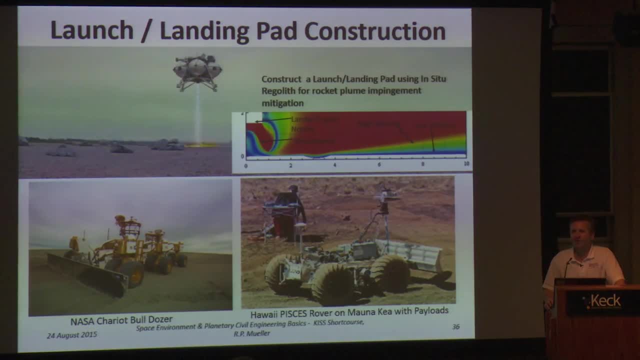 and patch the concrete and he's getting tired of doing it. So he came to us and he said we need to do better on the life cycle of these landing pads. The life cycle cost is too high, Too much work, So we have to develop this launch landing capability. 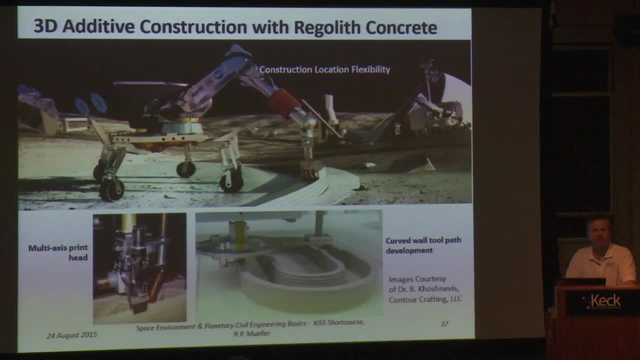 There's also been some unique work done by Dr Barok Kushnevis at the University of Southern California with contour crafting, And so contour crafting is a promising technology, but, you'll notice, it uses Portland cement concrete, which we will not have in space. 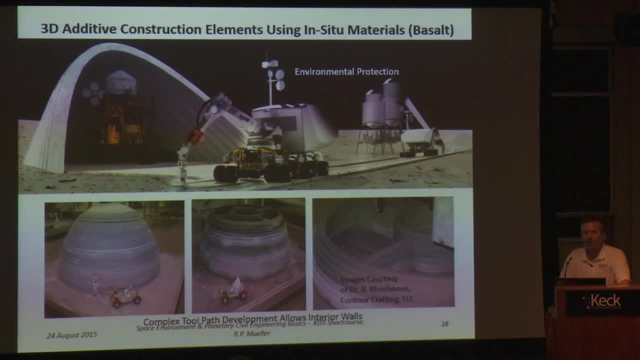 It uses a lot of water too, So that's really not an option for space materials-wise. but the basic technology is showing feasibility And Dr Kushnevis had some NASA contracts to go look at this. So Mars will have infrastructure. 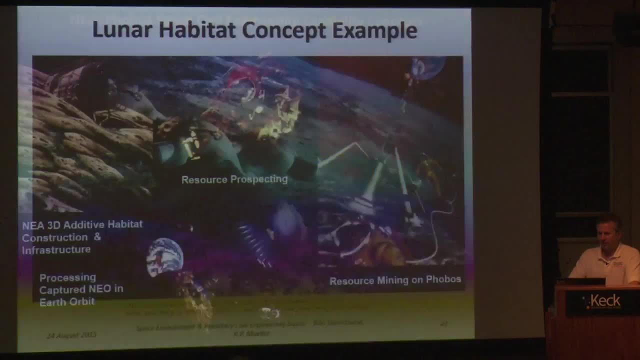 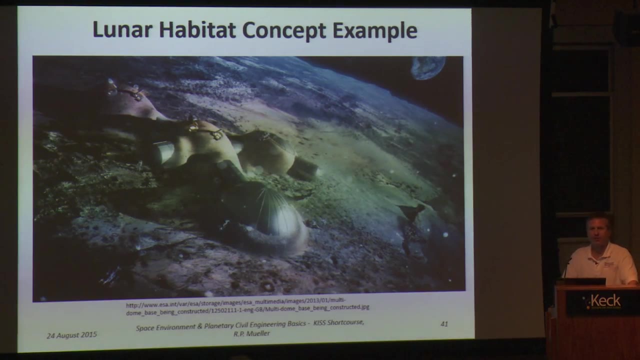 and asteroids will have infrastructure and the Moon will have infrastructure. This is a recent study by some of our colleagues at Foster & Partners- and they're here at this workshop- and also the European Space Agency funded this work And they came up with these very beautiful images. 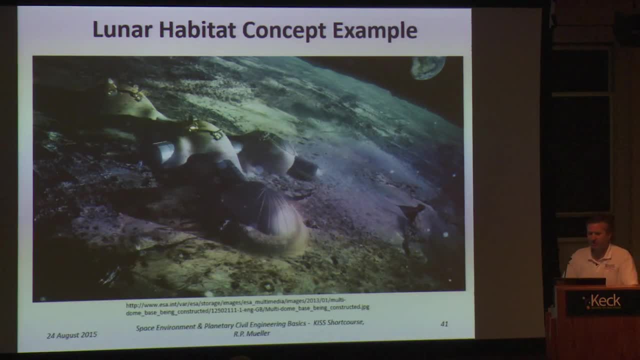 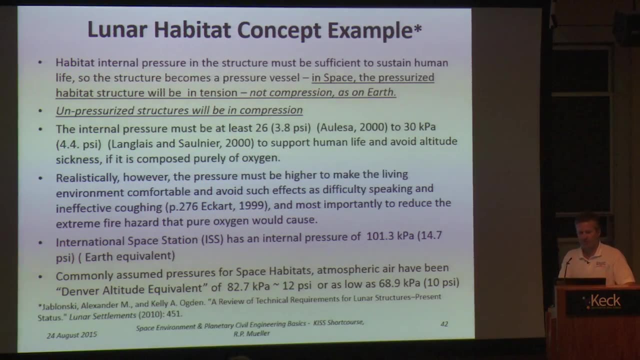 of what a lunar base could look like and this kind of graphic is starting to get in the right direction of what's realistic And the reason why- and I know there's a lot of words here, but the basic message I want to give you is that in space, the pressurized habitat structure will be in tension, not in compression. All the structures we have here on Earth are usually that use. concrete are usually in compression. The tensile strength of concrete is 10% of its compressive strength. It's a material that's very good in compression, very bad in tension. However, a pressurized habitat has to be good in tension. An unpressurized structure is okay if it's good in compression. The reason we use concrete on Earth is because it's cheap. 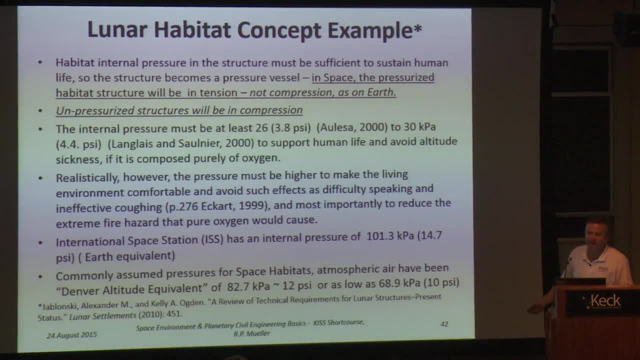 It's a cheap, very widely available material and that's why it's used, Because if we have a pressure vessel that we live in, what's the pressure? Well, so some literature says at least 3.8 psi, 26 kilopascals to 4.4.. That's pure oxygen. That's dangerous, That would probably cause a fire. So we don't want a pure oxygen environment. So what is the right pressure? Well, ISS has Earth equivalent 14.7 psi. That's what you and I are breathing right now. 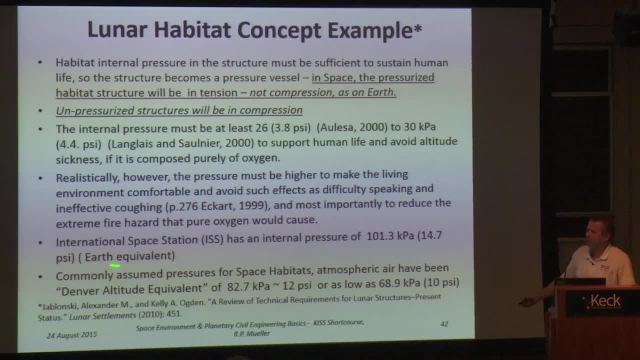 101.3 kilopascals, But that puts a big burden on the pressure vessel, 14.7 psi. So what we commonly assume is: let's say okay, let's say we live in Denver. In Denver, a mile high city. 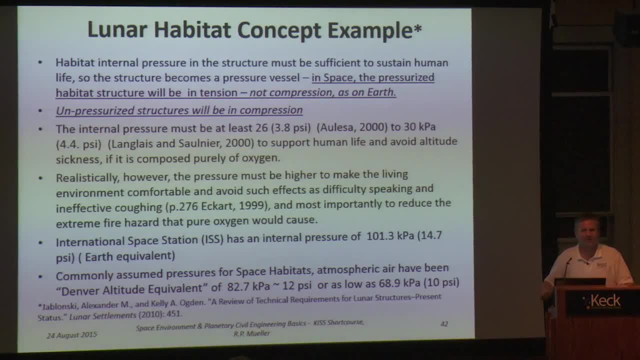 That's okay, right? People don't look weird there, They act normal, They're okay, So that's fine. So we say that is 12 psi. Living in Denver is 12 psi And we can go as low as 10 psi. 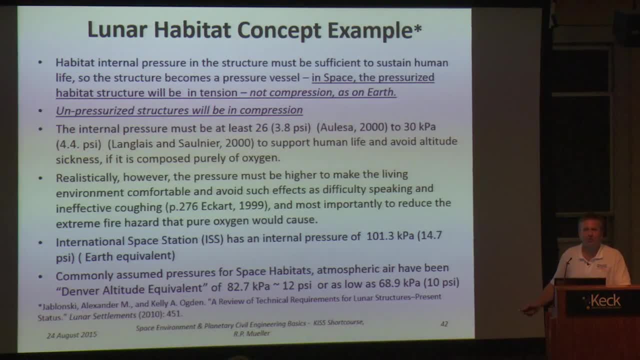 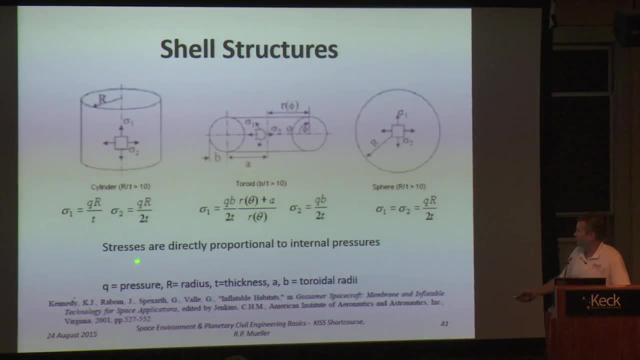 Say: you're living in the Himalayas, You're still okay. So we know humans can live in those kind of pressures. So we can go as low as 10 psi. Why does that matter? Because stresses are directly proportional to internal pressures. 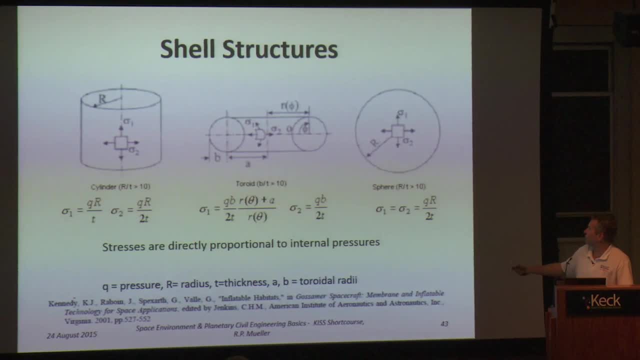 These are kind of notional habitat shapes. You could have a cylinder, You could have a toroid, You could have a sphere, You could have a combination of these, Like Transhab was a combination of a toroid and a cylinder. So the various combinations, basic messages. 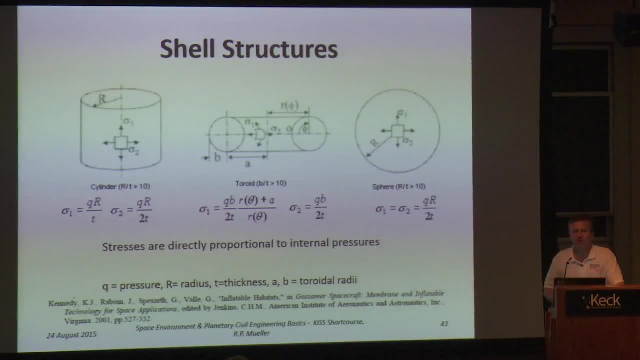 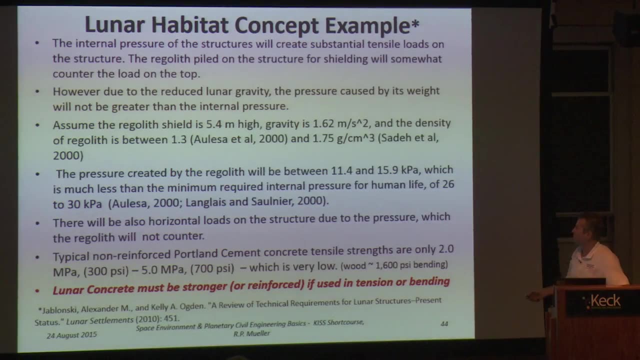 stresses are directly proportional to internal pressures, So you should try to minimize the internal pressure or come up with a solution that is not a pressure vessel. Now, the next thing in here- and I'm sorry for all this text, but this is all about trying to offset the internal pressure. by piling regolith on top of a structure. So let's say you have a pressure vessel pushing outwards. If you could pile regolith on top of the pressure and push inwards, you might be able to mitigate the effects and reduce the requirements on that pressure vessel. 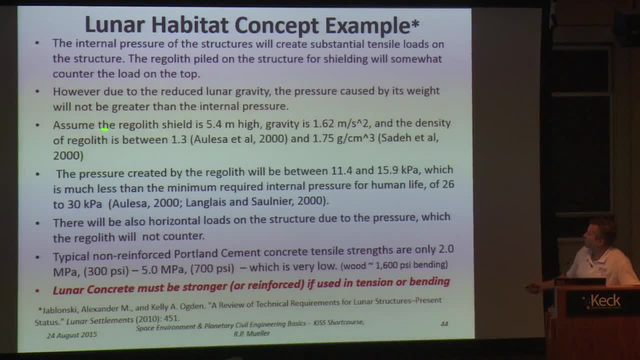 And so if you assume that the regolith shield is 5.4 meters high, then you're going to see that the density of regolith is between 1.3 and 1.75 grams per centimeter cubed. The pressure created is between 11.4 and 15.9 kilopascals. 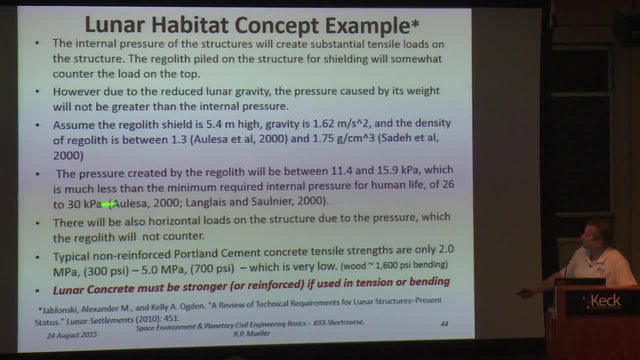 which is much less than the total pressure of 26 to 30. And this was at the 4 psi pressure of pure oxygen, which is not good for long-term operations. So really it's not enough. The message is: it's not enough. Piling regolith onto a pressure vessel is not enough to offset that tensile strength deficit, And so we have to come up with solutions for that Typical, non-reinforced portless cement concrete. it's only 2 megapascals. or 300 psi to 700 psi tensile strength. Just to give you an idea, wood is 1,600 psi bending, so it's 2 to 3 times less than wood. So would you build a pressure vessel out of wood? 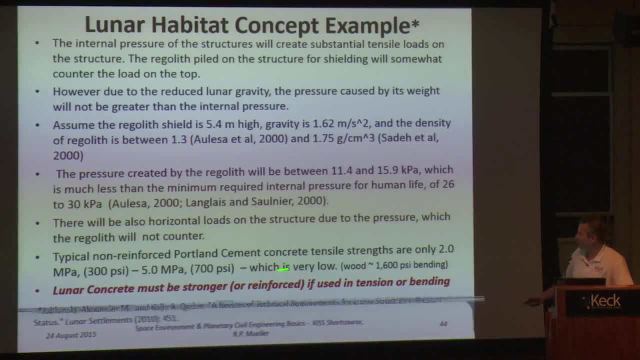 I don't think so, So it's a hard problem. Lunar concrete must be stronger or reinforced if used in tension or bending. So we have a materials issue And the next talk we have is going to talk about those materials. The next: 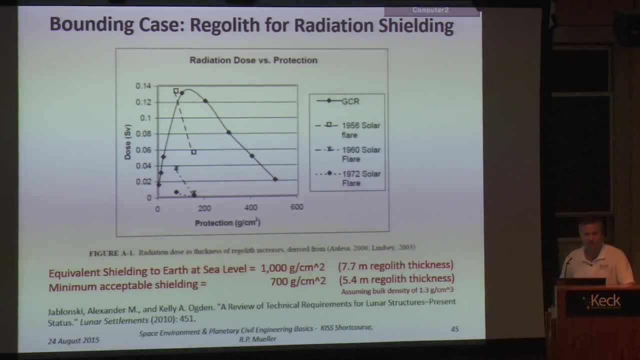 Well, I don't know. Okay, I think I touched the connector. The next really interesting thing is: people have been talking about putting regolith on habitats for radiation shielding. In fact, if you put regolith on a habitat for radiation shielding- 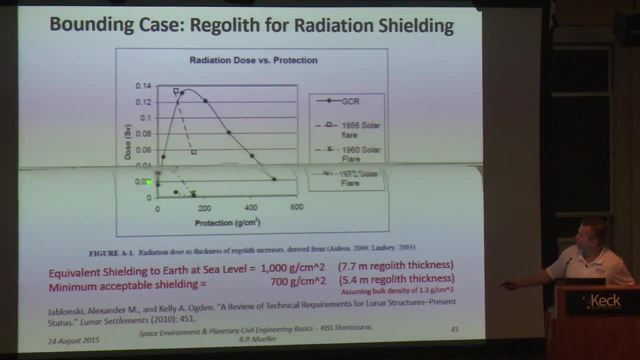 it's likely you'll make the problem worse. So right here you show, this is the density of the regolith that you put on And if you go up here, this is about one meter of regolith shielding here. This is the GCR, the galactic cosmic ray dose in Sieverts. 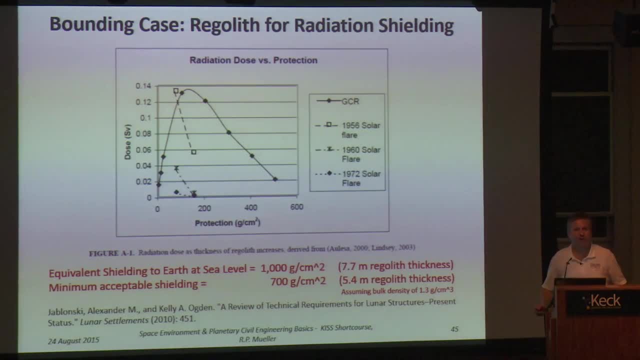 As you put more regolith on, it gets worse. The problem gets worse and worse. Why? Because of secondary radiation. The radiation comes in. these high energy particles come in, they hit the regolith mineral particles and eject more particles. There's a cascading effect. 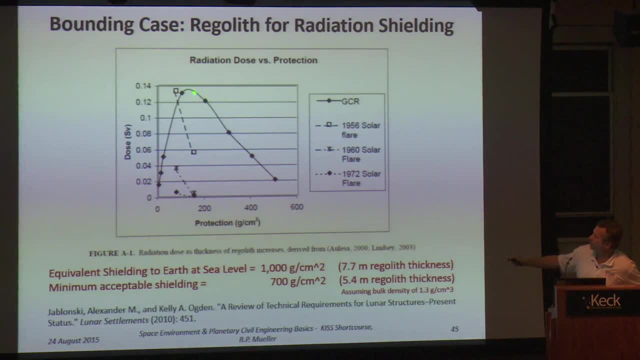 So it makes it worse And it gets worse and worse and worse. Then it peaks. here That's about one meter. Right here is about two meters of regolith, And then you're into three meters, And so the equivalent shielding on Earth. 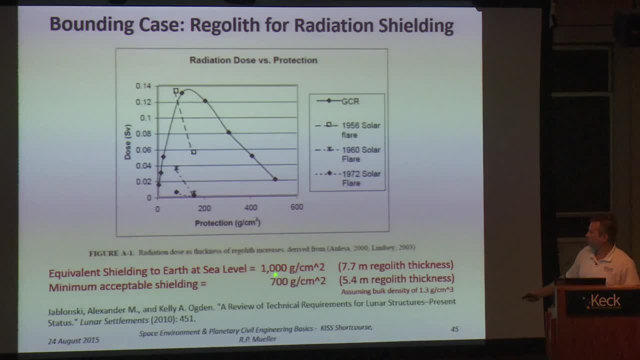 if you wanted to have the same radiation environment as you are on Earth would be 1,000 grams per centimeter squared. That equates to 7.7 meters of regolith thickness. So in order to get past here, this is 500 grams per centimeter squared. 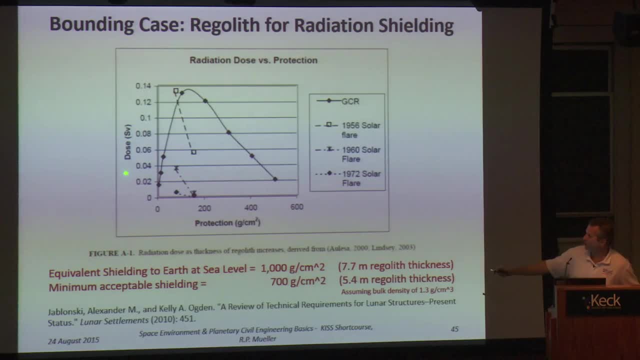 It's about four meters of thickness. Then you're back to where you were without having any regolith, And then you have to put more regolith on to get the shielding you need. So you need 7.7 meters of regolith thickness for shielding. 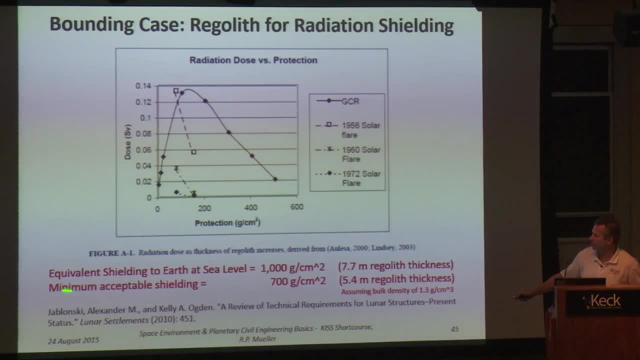 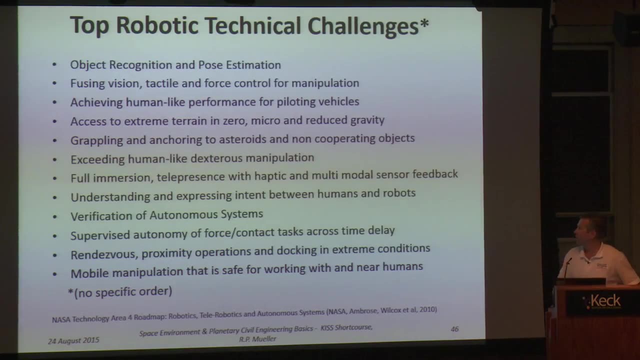 and 5.4 meters for minimum acceptable shielding, But it's a lot of regolith. Those are the kind of numbers we're talking about. Most people have been talking about one meter, two meter. It's not enough. I'm not going to get into this. 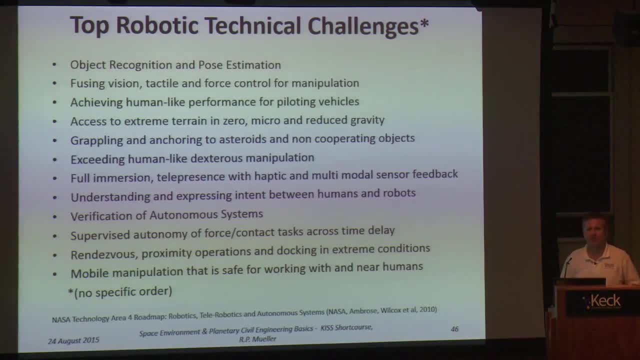 because Brian Wilcox has a talk later on to talk about robotics, And so we'll wait for that. But there are some challenges And these came from the NASA Technology Area 4 Roadmap. You can look it up. It's all listed in detail in the NASA Roadmap.